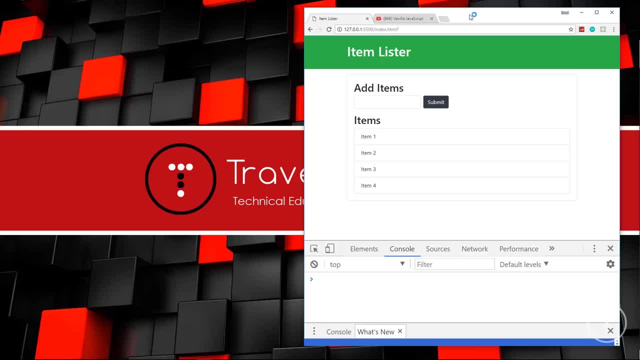 We're also going to just take a look at the DOM in general. We're going to look at all the some of the different properties of the document object And we're going to do a little exploring, And this is the page we're going to use to do it with. This is just a simple HTML page that I created that includes bootstrap, has some bootstrap classes just to make it look good, But it's basically just a header And then we have, you know, a card with a form and then a list group, Okay, and we have certain classes and IDs and stuff. So that's what we're going to do. 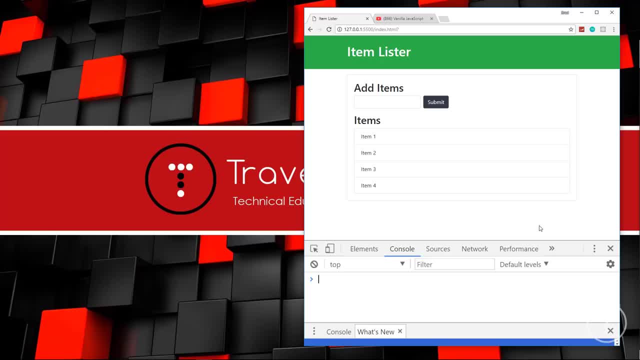 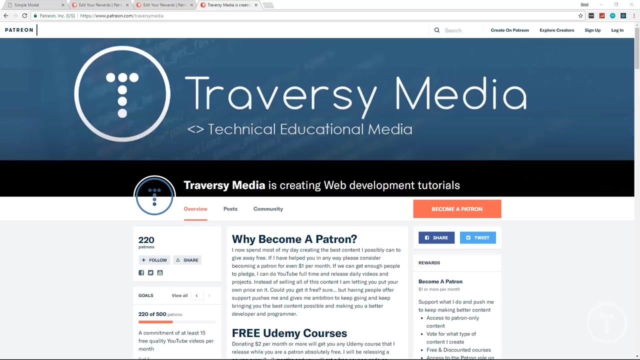 But we can select certain elements All right. now, in the description you'll find a link, and it will. it will include this, the bare HTML file, without any JavaScript, And then, as we move along, you can, you can code along with me and add the JavaScript. I'll also have the final versions of the code as well, All right, so let's go ahead and get started. So if you guys really enjoy my content, you feel like you really get something out of it, consider becoming a patron to push me to keep bringing you high quality education. 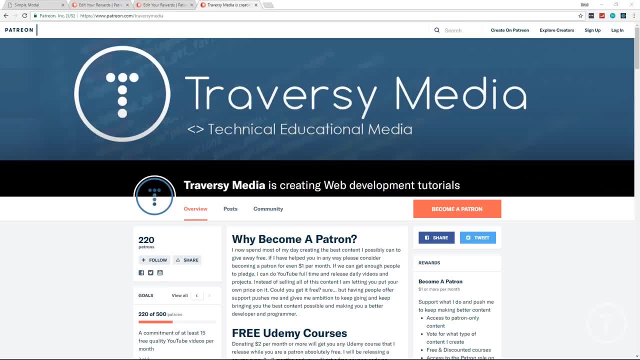 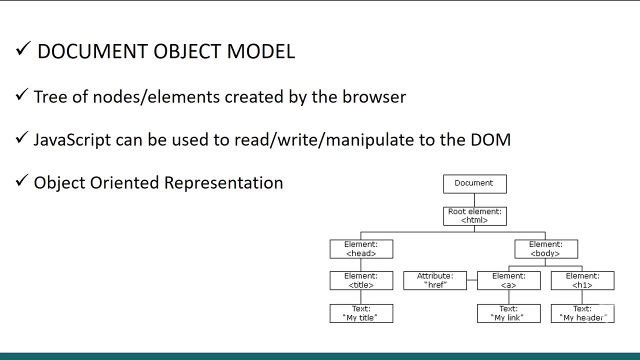 All right, so before we get started, let's talk a little bit about what the DOM actually is. So it stands for document object model And it's basically a structured representation of your HTML document. Okay, it can be thought of as a tree. 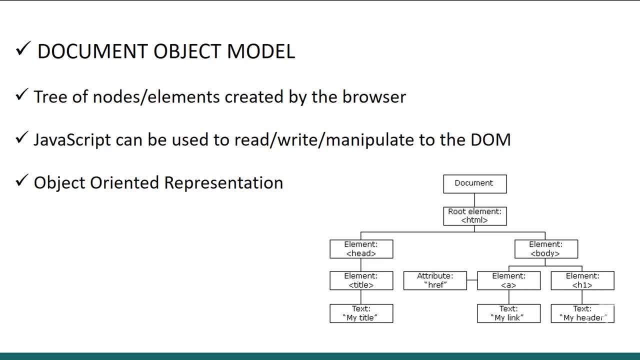 of nodes or elements created by the browser. JavaScript can be used to manipulate the DOM and its elements. The DOM is object oriented, meaning that each node has its own properties and methods that we can go and we can change and we can add, we can remove things, So we can manipulate basically everything on the page using JavaScript. Okay, jQuery was used to do this for a long time, but it's becoming more and more popular to use just vanilla JavaScript for this, And that's what we'll be doing. So you may have 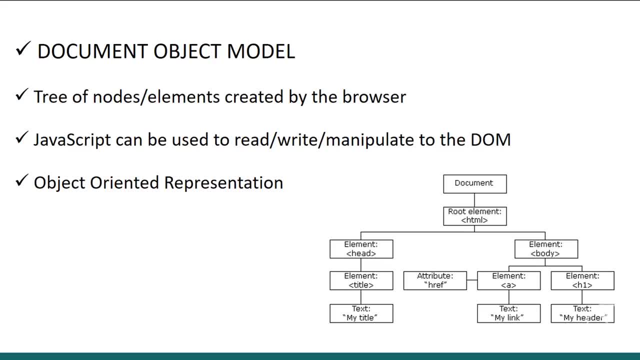 seen diagrams like this around the web. Now the browser gives us a window object which represents the browser itself, It's the top level object, And then we have a root element inside the document. Okay, so well, in the window we have the document object, basically the the core of the DOM, And then we have a root element which is the HTML tag or the HTML element or node, whatever you want to call it, And then inside that we have 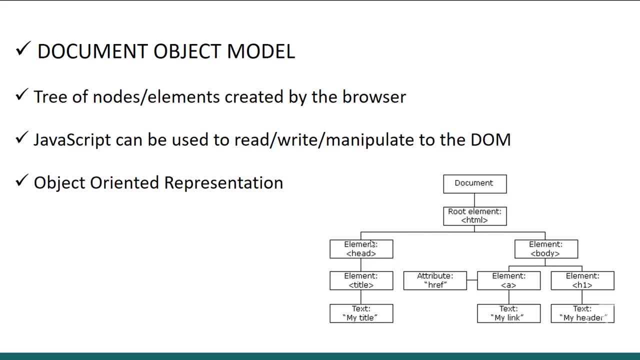 children, like head and body tags- okay, our head and body elements nodes, And then those have their own children. So we have a title. for inside the head we have titles, we have things like meta tags. In the body we have things like h ones and a tags and all kinds of stuff. And then those tags, those elements, they have text nodes. So, for instance, we may have an h one with the text of my header. that's also considered a node. We also have attributes, okay. 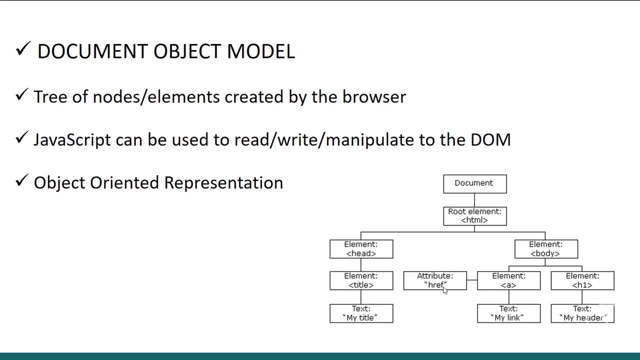 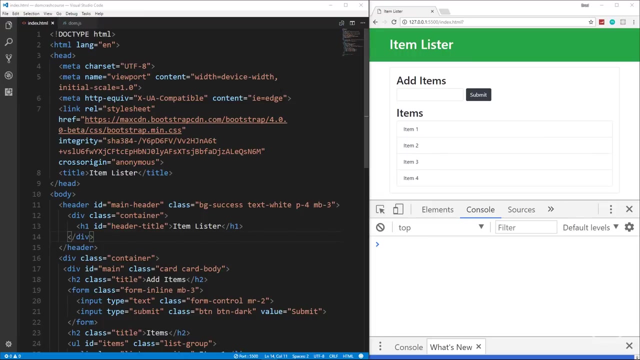 connected to elements. For instance, we have an h ref attribute on an- a tag, or an- a element. So this is, this is the DOM, Okay. all this stuff together, looked at kind of as a tree like this is the DOM. Okay, And we can manipulate this stuff with JavaScript And that's what we're going to do, Alright. so let's go ahead and do it, Alright, guys? So on the left here I have Visual Studio Code open. I'm using live server. If you want to use that, you can just click on it. 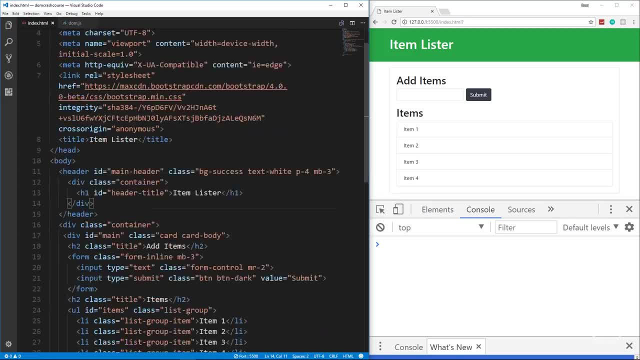 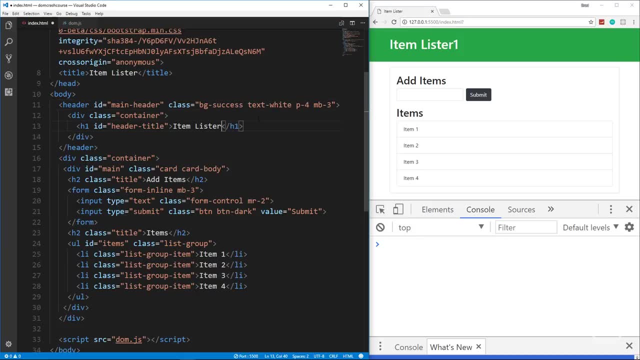 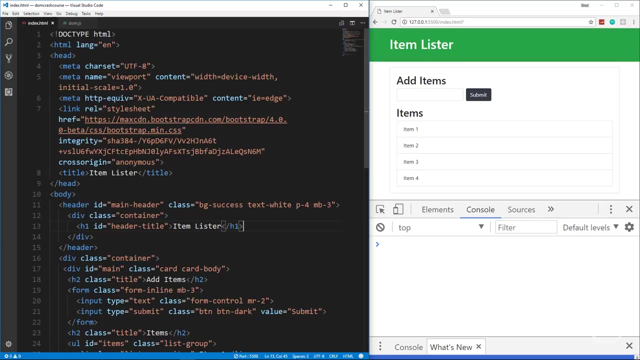 extensions and search for it and install it, And that'll make it so this auto loads every time you save. If I go ahead and I say item lister one and I save, you'll see that it'll auto load, Alright. so if you're not using an extension like this or atom live server or something like that, then you just have to reload, Alright. but let's go over this real quick. So it's just an index HTML file. This is going to be included in the description, okay, and a link in the description, And we just have a link to bootstrap, to the CDN, to 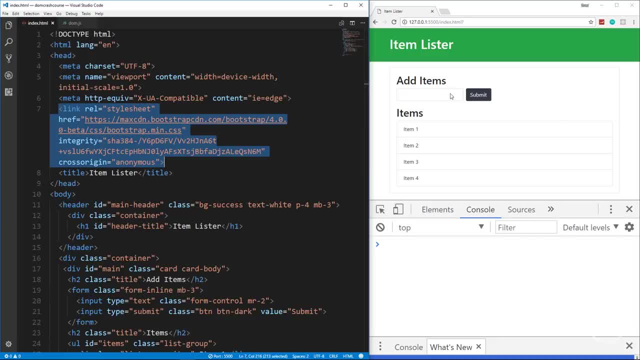 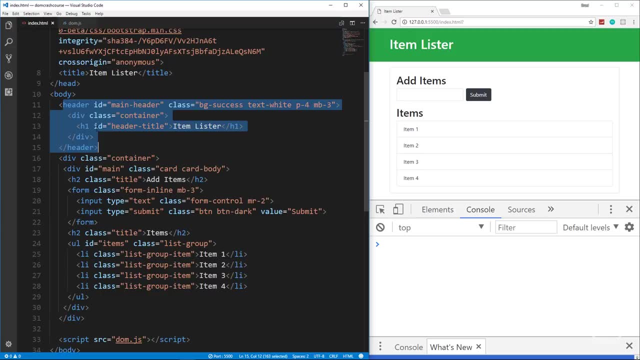 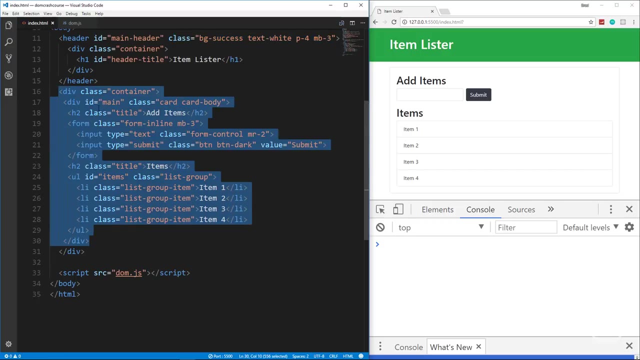 version four, But this doesn't really matter, I just wanted to use it to kind of give it a nice style. Then down here we just have a header. Inside the header we have a container with an H1, with an ID, where you have some bootstrap classes. Then we have under the header a container, we have a div with the ID of main class of card which gives it this border around it. And then we have an H2, a form with one field and a submit button, And then we have an H2.. And 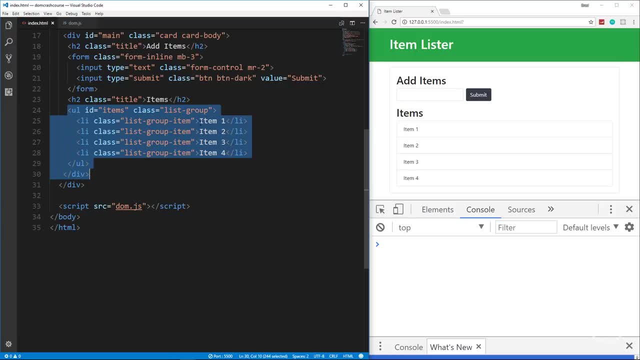 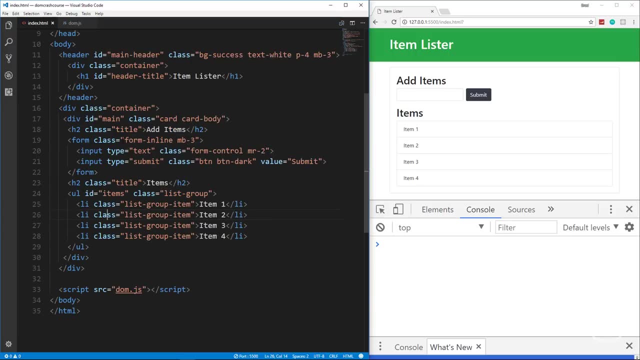 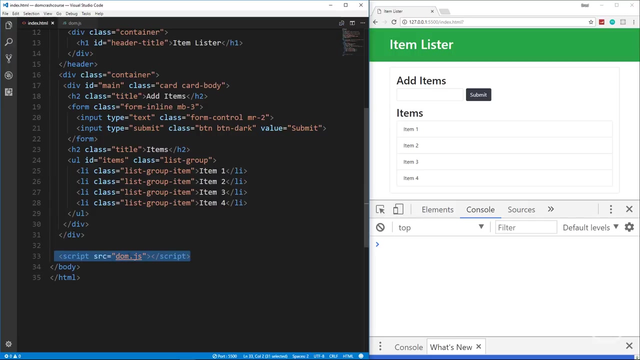 then a UL with the ID of items and the class of list group, Okay, and each list item has a class of list group item. So that's the DOM. that that's the, the HTML structure that we're going to be working with. we will be adding and removing a couple things, But this is going to be the basic page that we work with. Alright, now down here we have a script point are pointing to a script called domjs, which is right here and is completely empty, And that's what we're going to be working with. 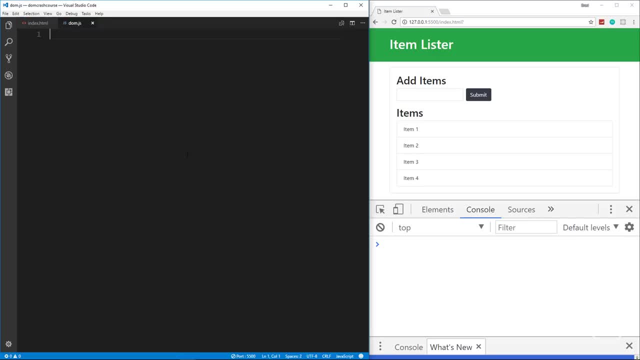 Alright, now, guys, I'm going to be moving a little fast here because this is a crash course, But I'm going to go over the the most important things as well as I can. Okay, so what you want to do is you want to have your console open, So you want to either hit F 12 or go to your your tools. you can go to your developer tools. The console is also available on other browsers- Firefox, Safari, whatever you're using- because we're going to use this for our output for a while, Alright, and then, once we get 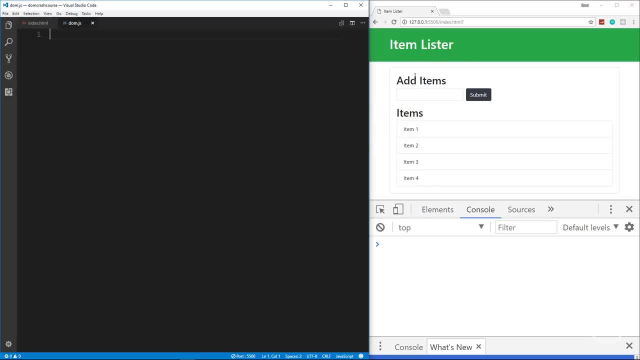 into actually changing things in the DOM. we'll be able to change text and styles and all that, Okay. So the first thing I want to do is just kind of examine the document object, Okay. so remember, in that diagram I showed you, the document is at the top And then under that we basically have a tree of elements So we can actually type in the console here JavaScript. if I were to say alert one, it'll actually execute that JavaScript. In fact, everything that we 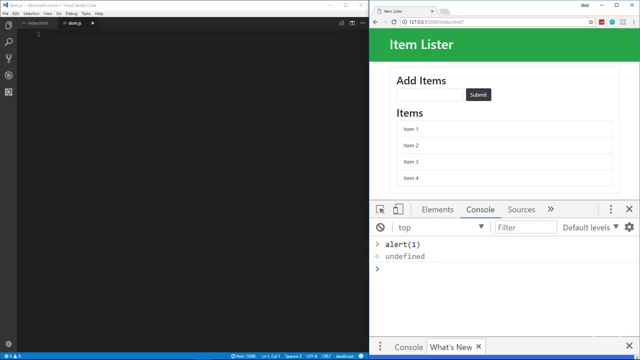 do in our file here. we could do in the console, But I want you guys to have this as a reference, Alright? that's why I'm doing it all in the file here. So what we're going to do is we're going to. 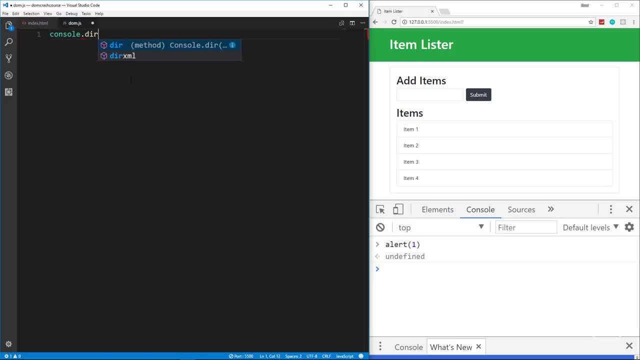 say, console, dot, dir, And we're going to pass in the document object. Okay, so what this is going to do is it's going to show us all of the different properties and methods attached to the document object. Alright, so you can see, we have like the URL we can access. 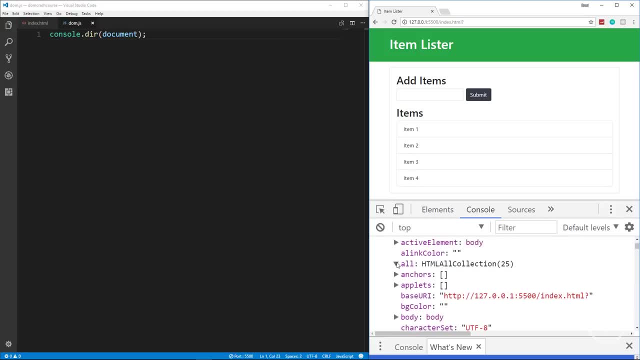 we have document dot all, which will give us an array- not an array but an HTML collection of everything that's inside of that page, that's inside of that document. There's the document dot body which we can access, and all the properties of that. So this is a very large 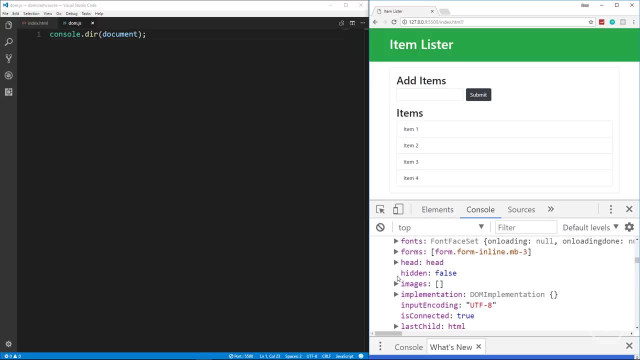 tree of properties and methods. I'm not going to go through all of this stuff, But I do want to show you some of the useful stuff. So let's go over here and just we'll just comment this out And let's look at some of the stuff that we can access through the document. Alright, so let me put. 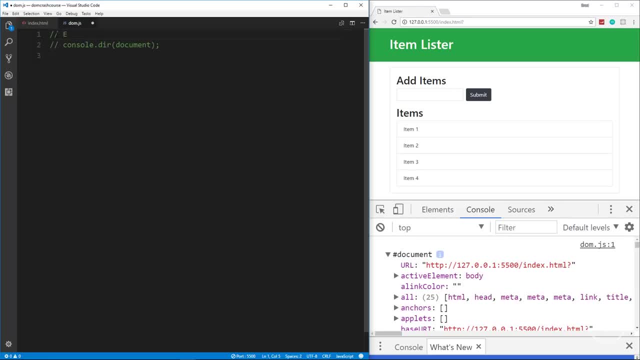 a comment up here And we're just going to say examine. we'll say examine, the document objects Alright, And you guys can use this stuff from within your scripts. When you create a JavaScript program, you can, you can access this stuff, you can edit it. it's not read only if you want to. 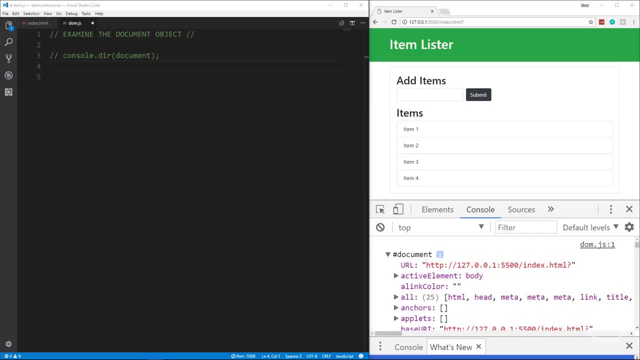 do that. So let's take a look at. let me see. first of all we'll look at the domain. So we can say console dot log, we can say document, we can use our dot syntax and we can access any of these. 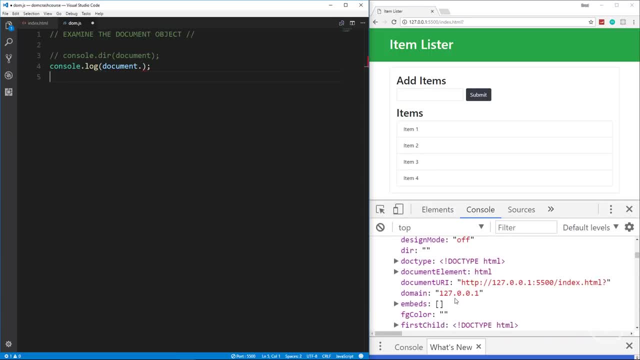 properties. So you'll see that there is a where is it domain right here which is going to give you whatever domain name you're running. So we say document, dot domain and save. you'll see that we get 127001.. Which is just basically my local host. that's the loopback address. Alright, we can also access the. 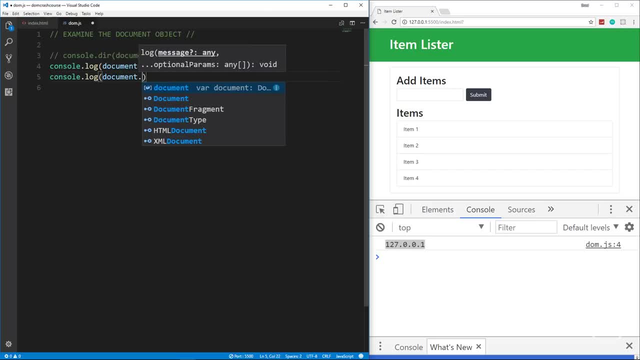 URL. So we'll say document, dot, URL and save, And it gives us basically the entire page and the entire URL. Alright, Another thing, you know what? I'm just going to copy this, because we're going to be doing this quite a bit. 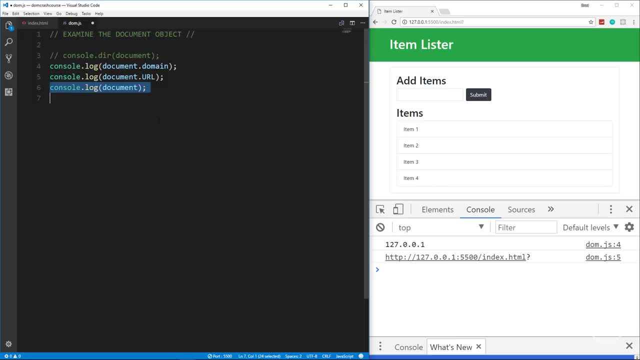 This console log. Another thing we could look at is the title of the page. So we'll say document dot title and we get item lister And you'll see the title is item lister. If I were to go and change the title over here to, let's say, 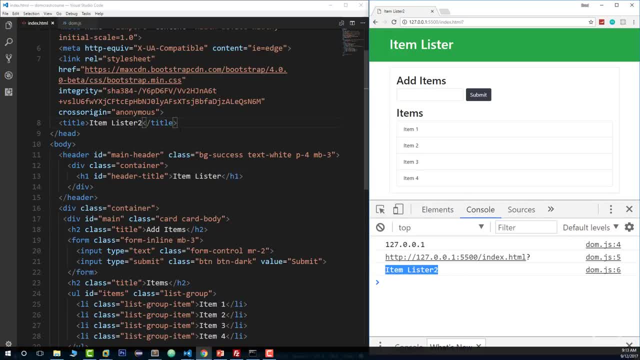 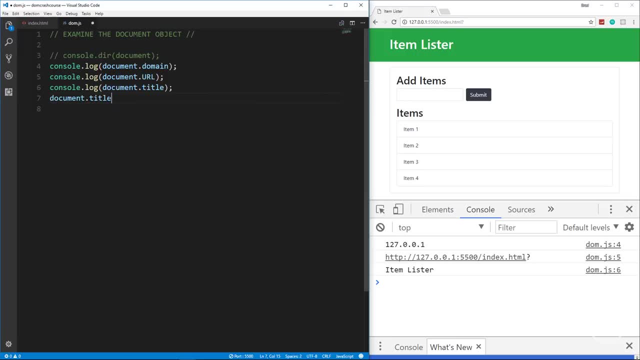 item lister two and save. now you'll see that that has changed as well, And this stuff is not just read, only we can change it. we could say document dot title, And we can actually set that equal to, we'll say 123.. 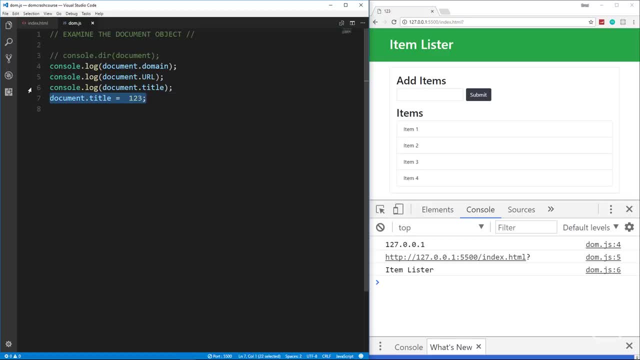 And now you can see the title has actually changed, So you can change this stuff from your, from your scripts, Alright. so another thing we can look at is: let's see, let's look at the doc type. So if we say dot, doc type and save. 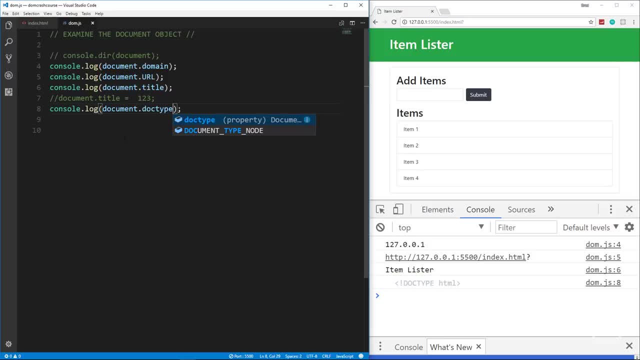 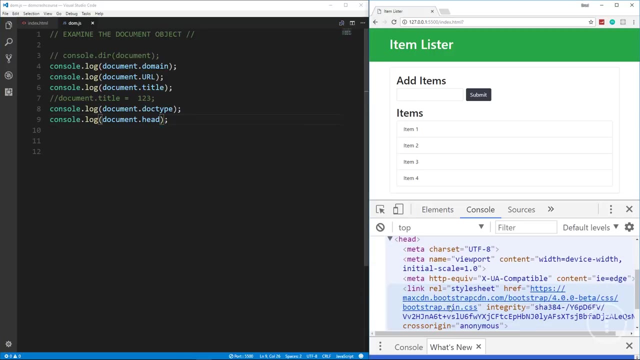 you'll see that we're using- excuse me, we're using- the HTML5 doc type. Alright, so we can also look at the. let's see the head and body. So if we say document dot head, That'll, that'll grab the head element and we're outputting it to the console And you can see everything that's in the head. 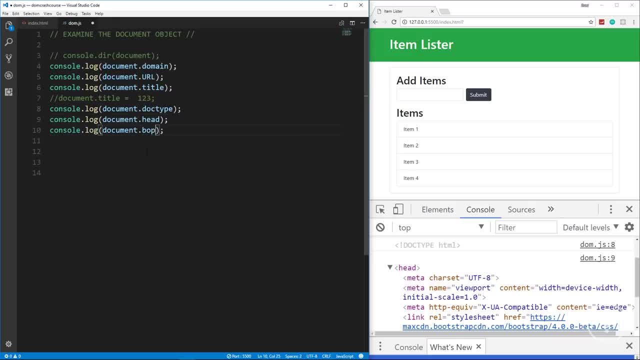 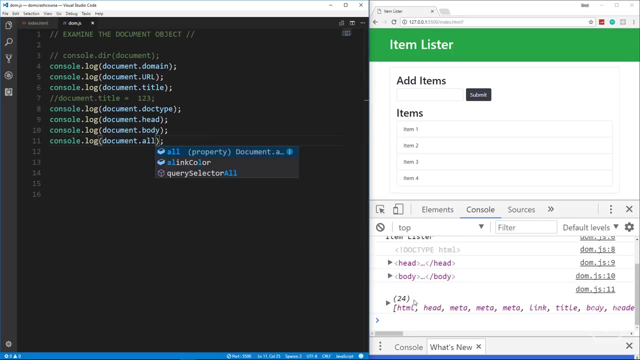 And, as you could probably guess, we can also do document dot body, which will grab the body for us and output it Alright. so another thing we can do is document dot all. So if we do this, what it gives us is an array or an HTML collection of everything that is in the DOM. So if we go over and we 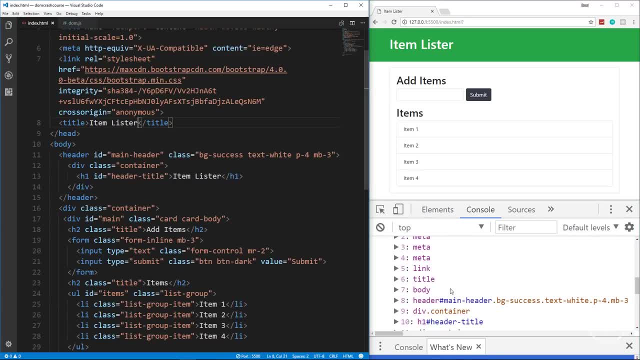 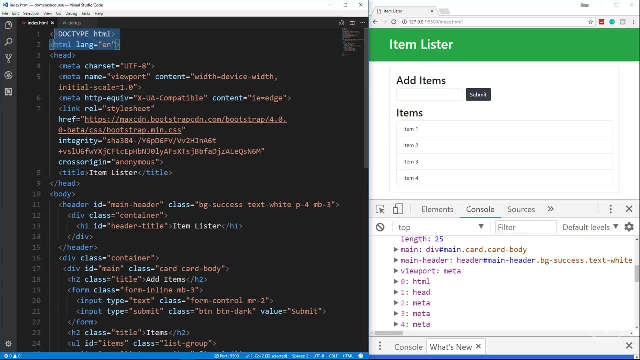 look, let's look at our index HTML file. you'll see if we go, if we start right here at zero. we have our HTML tag, which is up at the top, Okay, and then the next one in the one index is going to be the head. then we have the meta, we have another meta. 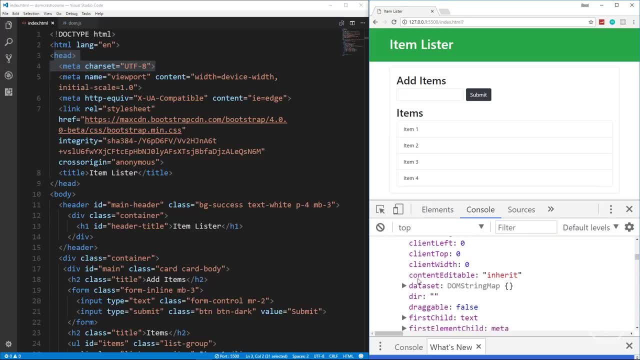 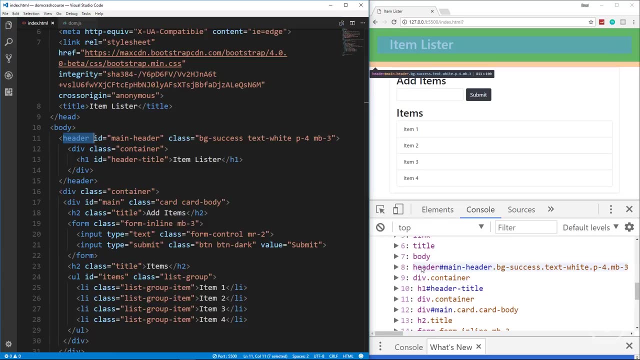 Okay, and if we open this we can see all the different properties of each of these elements. Okay, so we can get pretty much anything we want on that element And if you go down you'll see the link: okay, title. then we have the body, then we have the first element in the body is the header you can see. it also has the ID in the classes. then we have the container, then we have the title. so we can access any of these. okay, and we can specifically access them by their index. 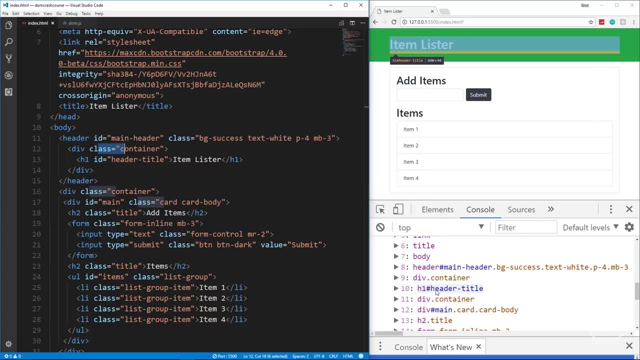 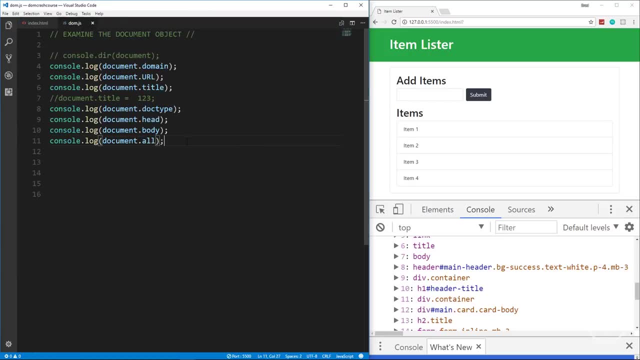 So, for instance, the header title, you'll see as I hover over it. it'll it'll, it'll highlight it in the browser. Let's say we wanted to grab this and it has an index of 10.. So what we could do is we could go down and we can see the title and we can specifically access them by their index. 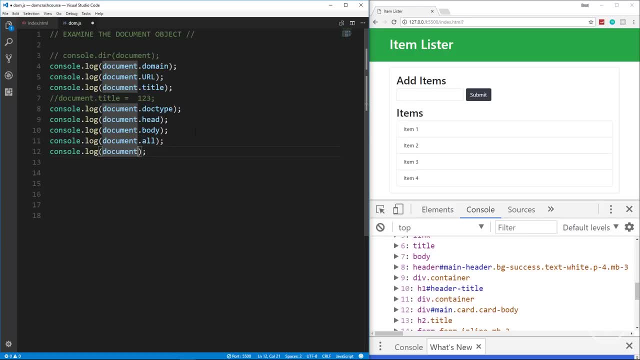 So what we could do is we could say console log, document, dot all, and we could grab the index of 10 and save, and it'll actually give us that H1.. All right, now again we can change things based on our selector. 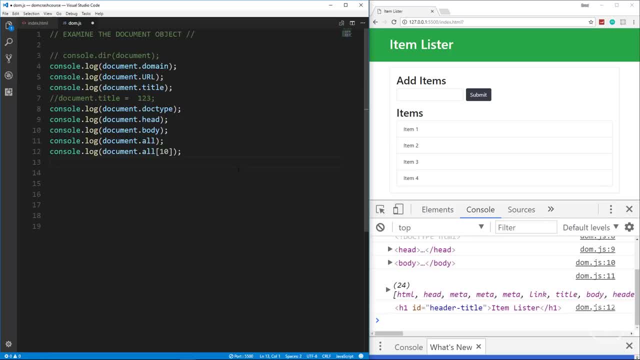 Now, this isn't. this isn't the way that you want to select things. I'm going to show you the specific methods for selecting things. but you could say document dot all and then grab the 10,, the index of 10, and say dot. text content equals hello and save, and you'll see that it actually changed that in the page. 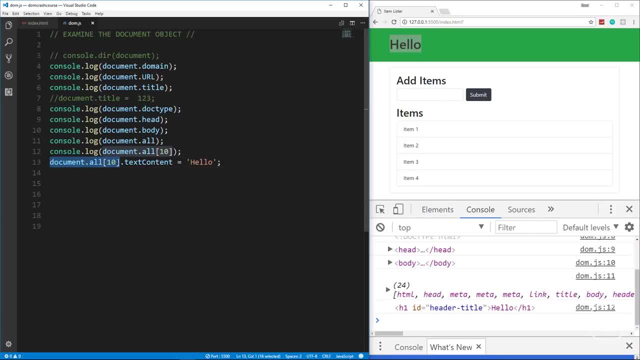 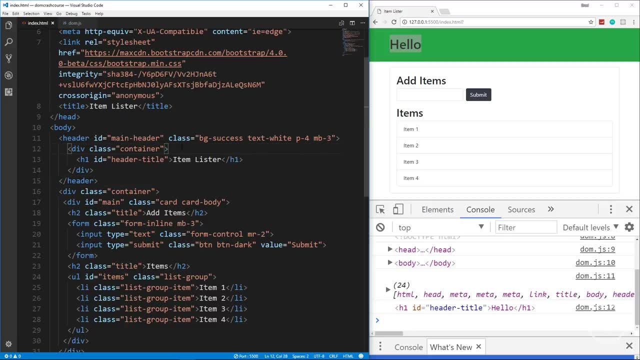 But this, this is not the way that you want to select things. All right, for one thing, if you add something, this 10 is going to change. If I go, and I go before that, and let's say we add a span and we'll just put like a one in here or something, 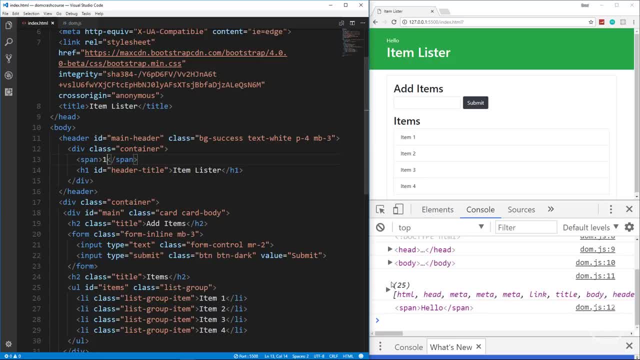 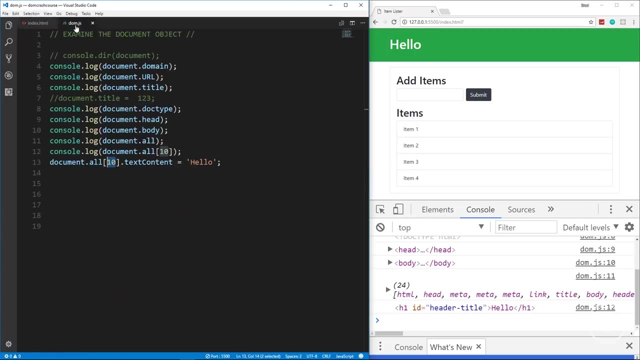 And save. Now that span is now the 10 index and that's what's hello. So you don't want to use that method of selecting from the DOM. All right, just to let you know that. And anything you add into your file here, whether it's in the head or body, it's going to get added to document dot all. 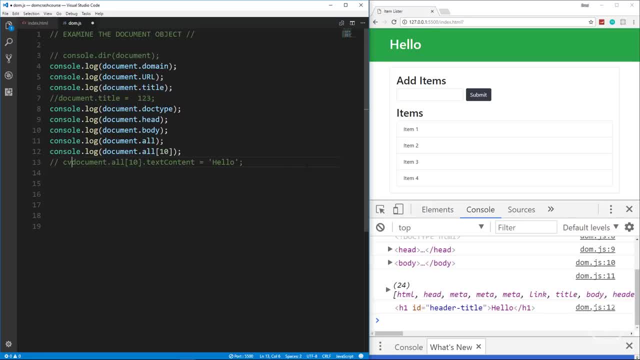 It's going to get added to that collection, All right, so let's see what are some other things we can look at now. Let's say you wanted to get all the forms on the page. You could say: let's do console, log, document, dot forms and save. 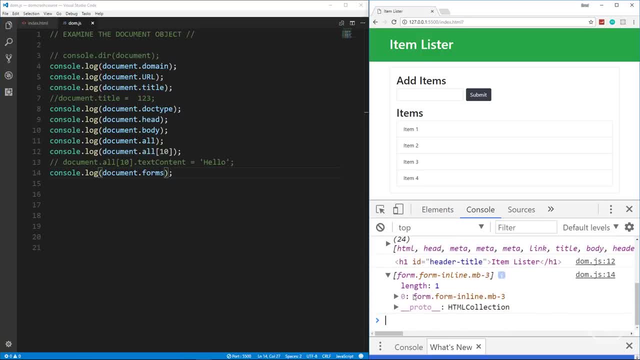 And we're looking right here. If we click this arrow, it's basically going to be a collection of all the forms. We only have one, so we have in the zero index. Okay, these always start at zero, just like a regular array. 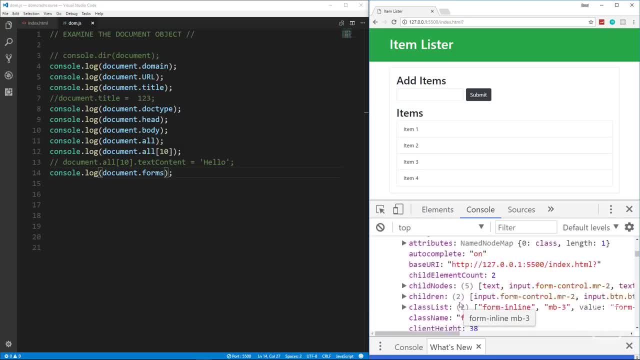 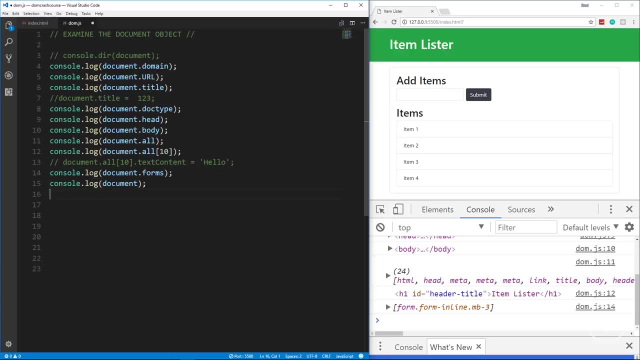 And then we have our form And you can get all the different properties of the form. All right, now you can do the same thing with like links. So if you wanted to get all the links on your page, you could say document dot links. 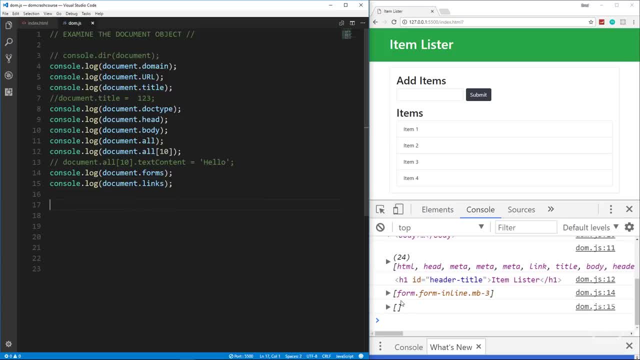 We don't have any, so we just have an empty array. I say array, but it's actually an HTML collection And there is a difference. There are things like, let's say, you wanted to use dot reverse, which is an array method in JavaScript. 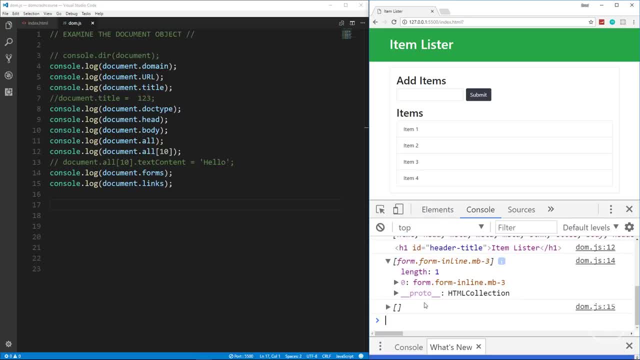 You couldn't do that, You'd have to first change it into an array. Okay, but you can select items like it's an array. Okay. Now, if you wanted to select a certain Item, like in our form, we have our zero index. we could say forms zero, like that, and it'll give us that actual form. 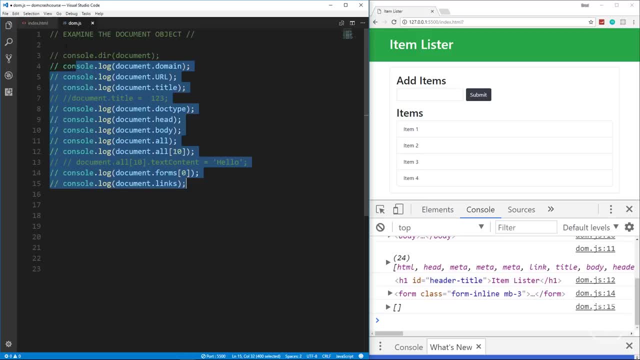 All right, so hopefully that that makes sense. I'm going to just comment all this stuff out so that this doesn't get too confusing. So what else? And in addition to links, we could do images, so we can say document dot images and you can get those. 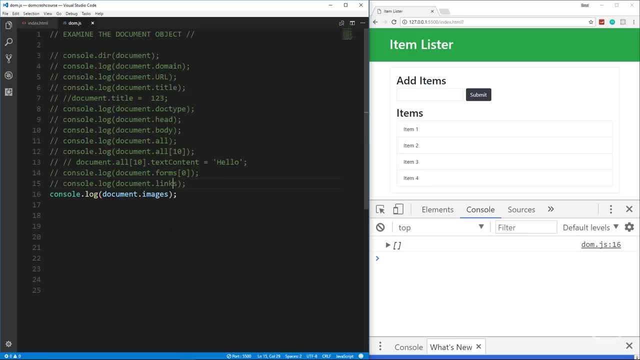 We don't have any, so we're going to get an empty collection. What else? I think that's it. I mean that's not it. Definitely There's more to it. You saw when we did console dirt document. there's a lot of different properties but I'm not going to go through them all because we'll be here all day. 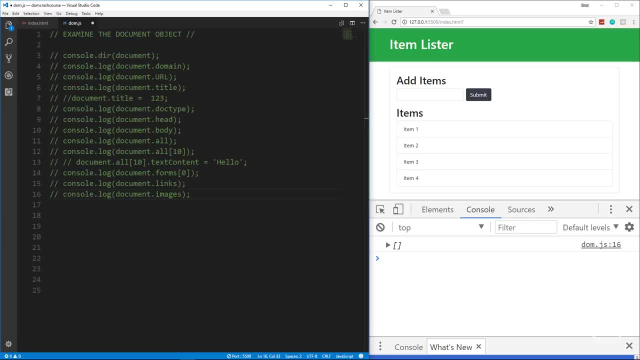 But those are some of the interesting ones. So what about selectors? Okay, So basically we have a few different selecting methods we can use to query the Dom. So the first one we're going to look at is get element By ID, which I'm sure you've heard of. 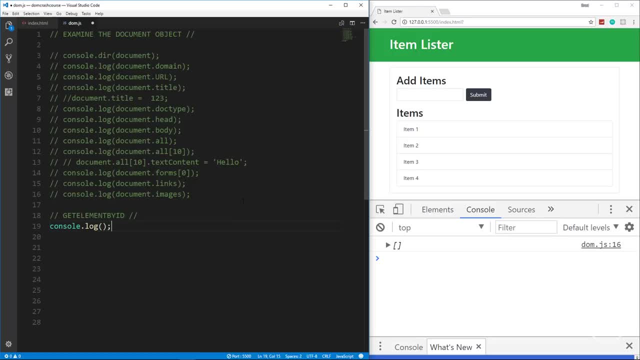 So what we're going to do here is let's console dot log and let's take a look at our Dom or our structure here And we have an H1 with the idea of header title. So what we'll do is we'll say document dot get, element by D. 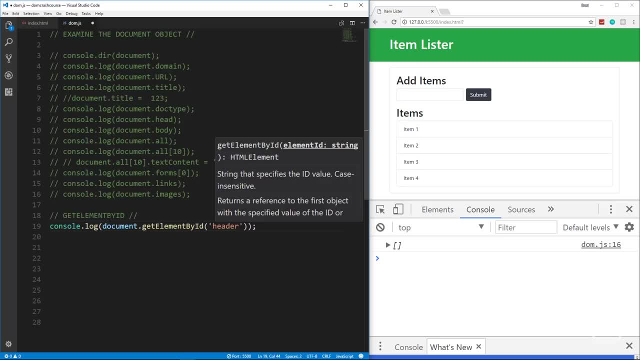 And we know that it has an idea of header title. Was it header title or no? header dash title: Okay, so if we save that, you'll see that it'll actually pull it from the Dom and we're just logging it. We can also put it inside of a variable. 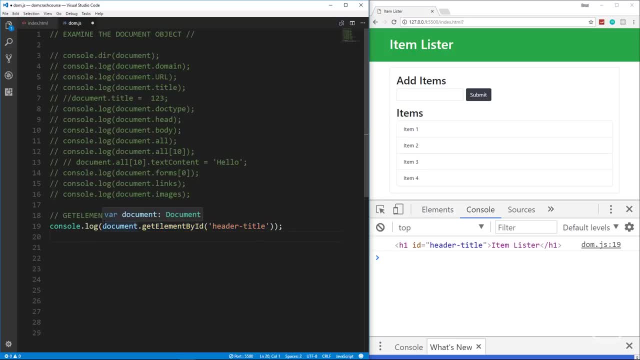 So if I copy this and we say I'm just going to use the five syntax, so we'll say VAR and we'll call this header title equals and then we'll paste that in and save and actually let's, let's log it So, header title save, and you'll see, we get the same thing. 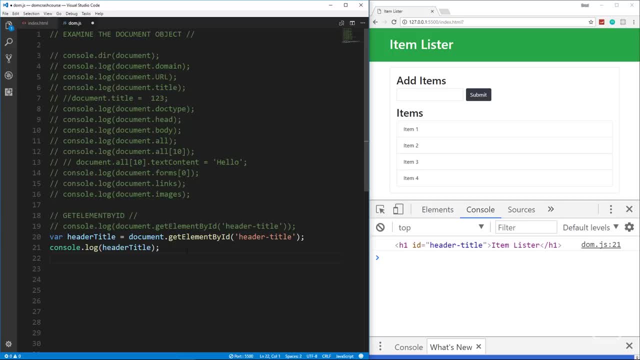 Now we can do certain things with this header so we can change the text. So there's certain methods we can use, such as text content, And we'll just set that to hello save and that'll change it. Okay, In addition to text content, we also have inner text. 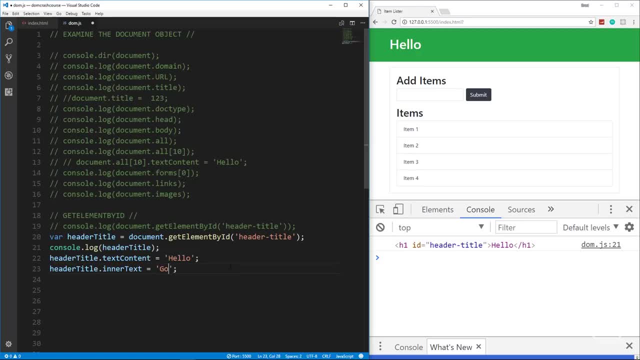 Which, for the most part, does the same thing. Let's set this to goodbye and save and you'll see it change, because we basically just overrode it. We overrode this with this. Now, the difference, or one of the differences, between inner text and text content is. one of them. pays attention to the styling. 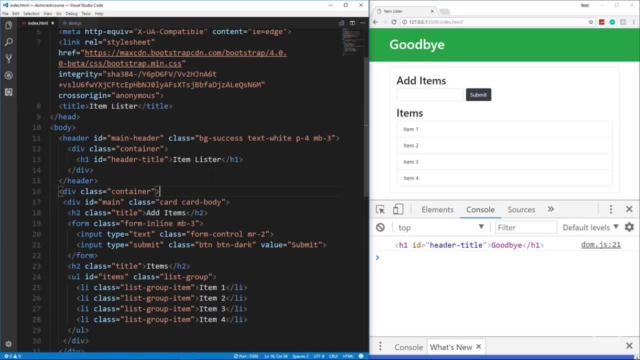 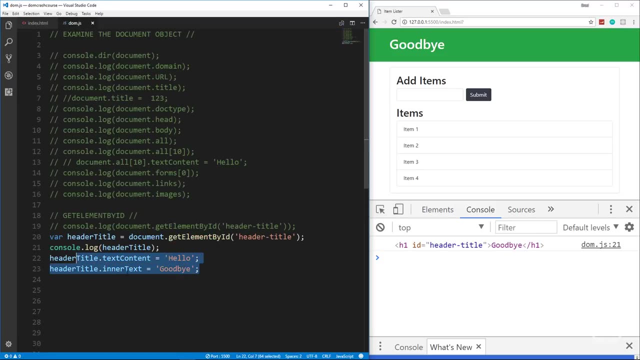 So let me give you, let me show you what I mean. So if we go into our H1 here and we put in a span And we'll just say I don't know, one, two, three, and we'll save- actually this is going to overwrite that, so let's just comment those out. but we get item list: or one, two, three. 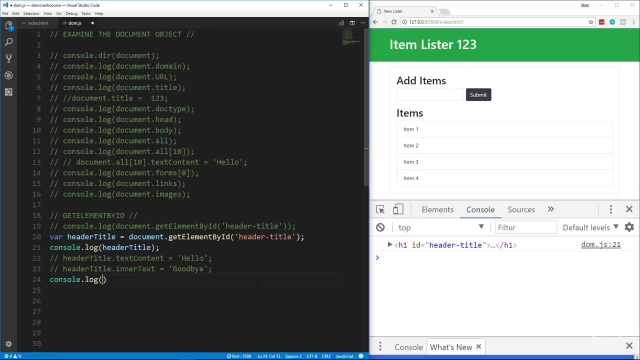 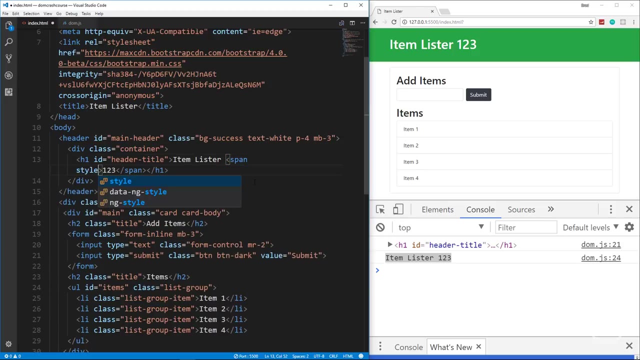 Okay, so let's go ahead and console log. header title, dot text content. All right, so we get item list or one, two, three. Now if I go to this span- And I had a style to it- Of display none. 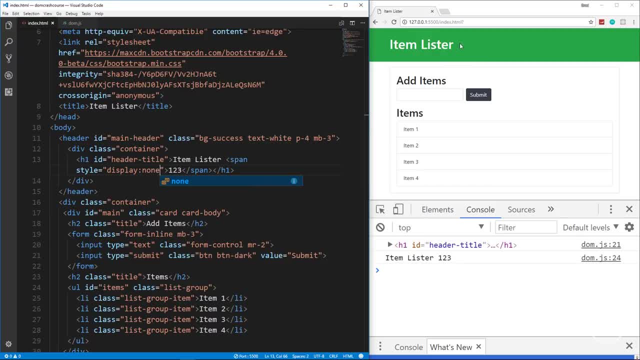 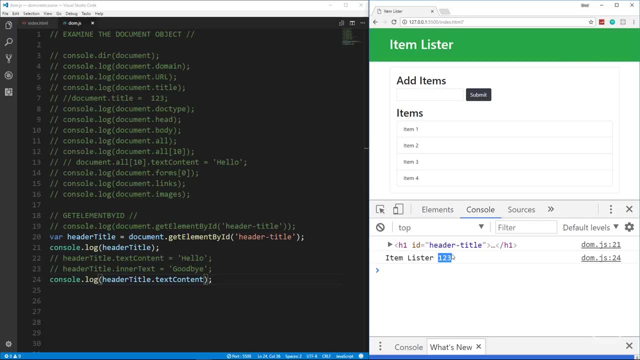 Okay, In the dawn and in the page here it's going to disappear, It's going to go away. now Text content is still showing the one, two, three. It's, it's, it's disregarding that span, even though it's set to display none. 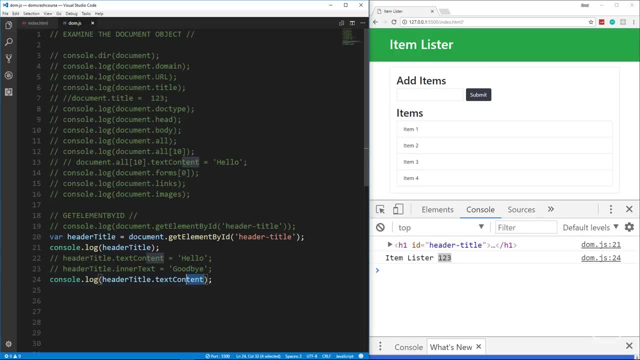 It still shows it here, But if we were to change this to inner text And save, You'll see that The one, two, three is not there. Okay, so it actually pays attention to the styling. so that's one of the biggest differences between the two, but you can use them for the most part pretty interchangeably. 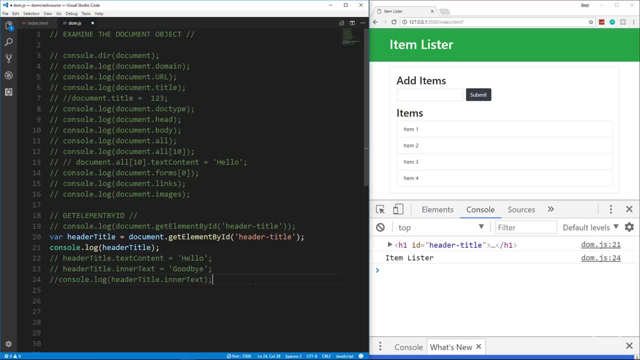 All right. So that's, that's what text content, inner text. We also have inner HTML, which I'm sure you guys have seen before If you've worked with JavaScript at all. So let's say header title And we'll say dot inner. 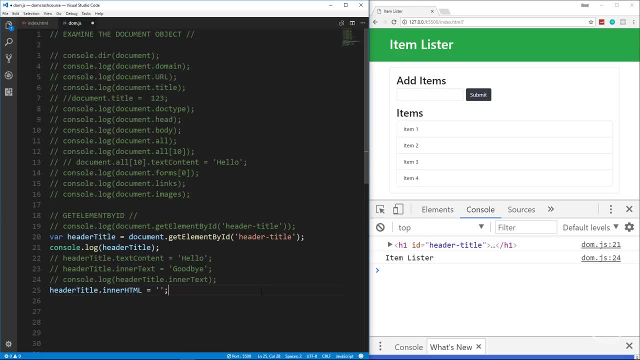 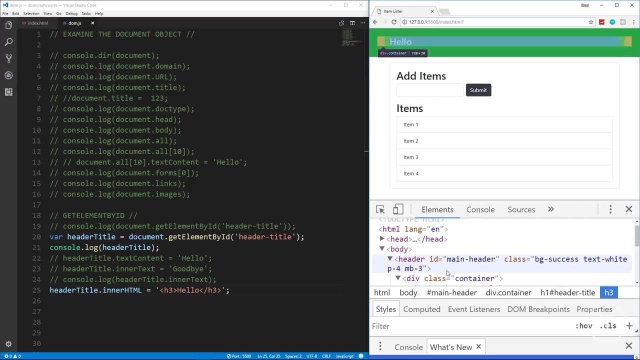 HTML equals: and let's put an H3. And we'll say: hello, save. Now you have an H3.. Now if we look at, if we look at it through the inspector, you'll notice that the H3 is actually inside the H1.. 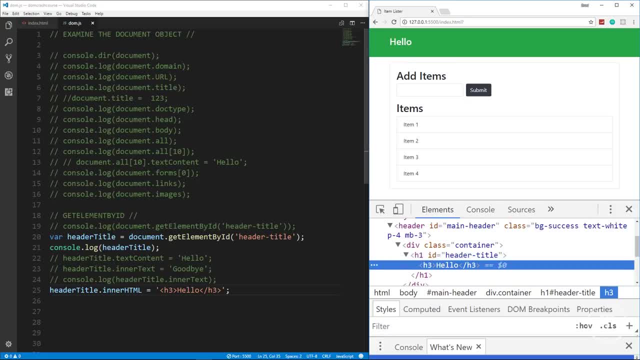 Now, it doesn't change the H1 to an H3. It puts the HTML inside of that, that DOM element. Okay, So that's what. That's what inner HTML does. Now, if you wanted to actually change it- the H1 to an H3, you'd have to use some other methods to access the parent element, and it's a little more advanced, and we'll get to that in a little bit. 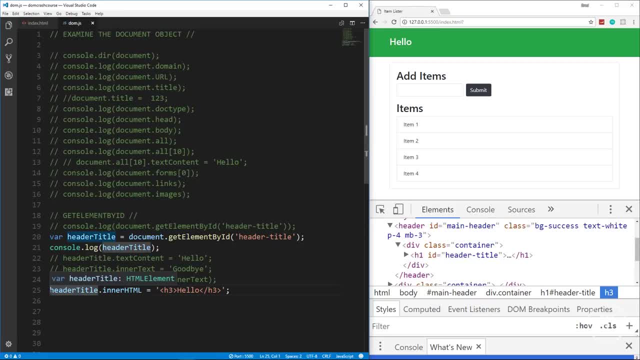 All right, But just keep in mind these, these three methods, So text content, inner text and inner HTML. Now we can also do style changes. Let's go ahead and save this, All right, So we just want to. I'm just going to comment this out too. 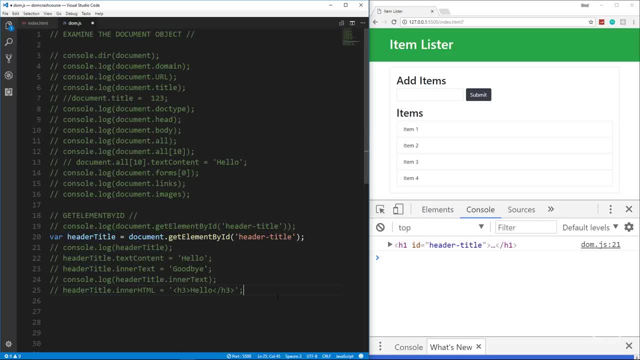 So basically we just have the header Title. So if we wanted to change the style like, let's say, header title and in all of these this text content, inner text, the stuff that I'm doing right now you can use with any selector, not just document dot. get element by D. 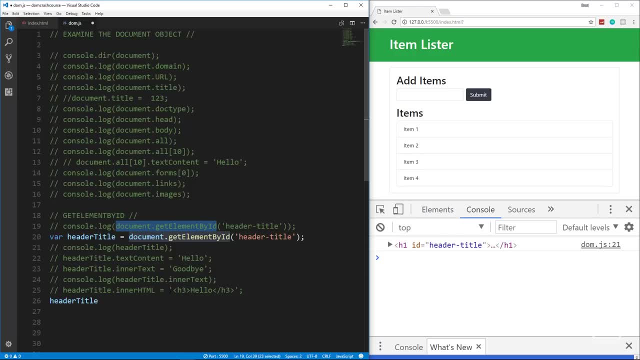 In fact, maybe I should have done all of the selectors first and then showed you this stuff. But you can use this with any, with any selector. Okay, Selecting elements and then using these methods are two different things. So let's say header title and we'll say dot style. 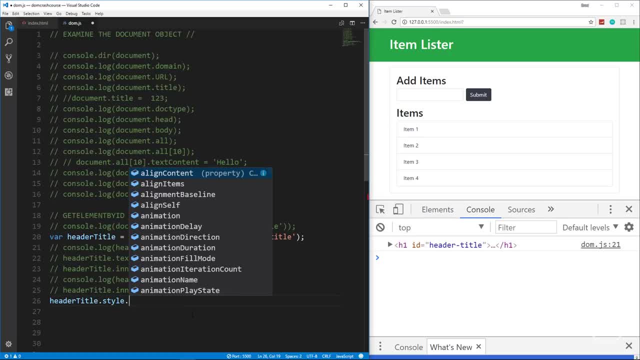 That's how you can change CSS styles. Let's say, we want to change the border bottom, All right. Now notice that I used camel case here, because you can't do border dash bottom, even though this is the the actual CSS property. 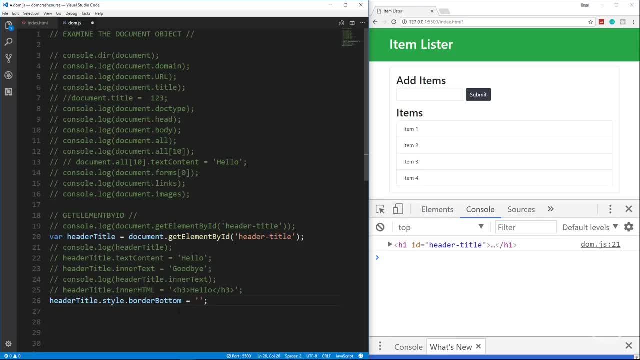 You can't do that, So you have to just change it to camel case. All right, So let's say we want it to be solid, three pixels And black and save, And now you can see that the H1 has the border. 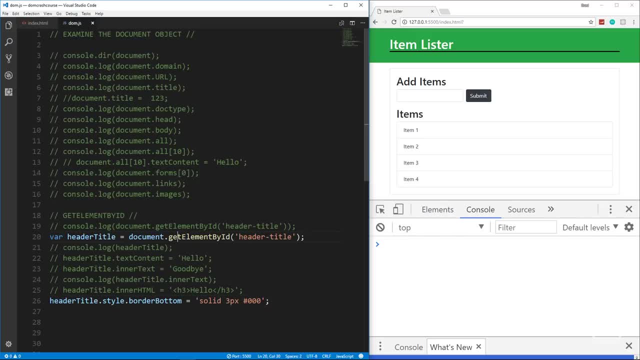 Actually I want to. I want to put that border on the header. So what I would do if I wanted to use get element by D. we know that the header actually has an ID of main header, So let's grab that instead. Or main dash header. 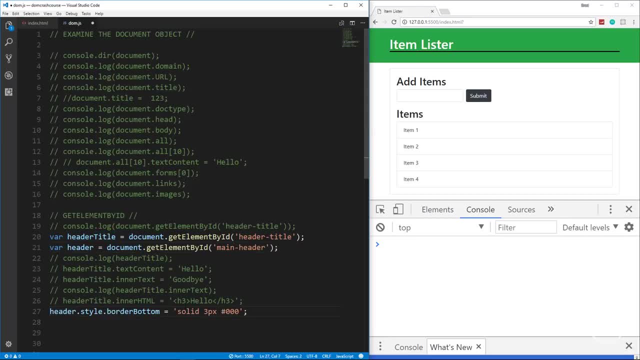 And then we'll just change this to header And save And now we have the border on the actual header. All right, So now you should understand to get element by ID, text content, inner text, inner HTML, and then changing the styles with style dot, whatever the CSS property. 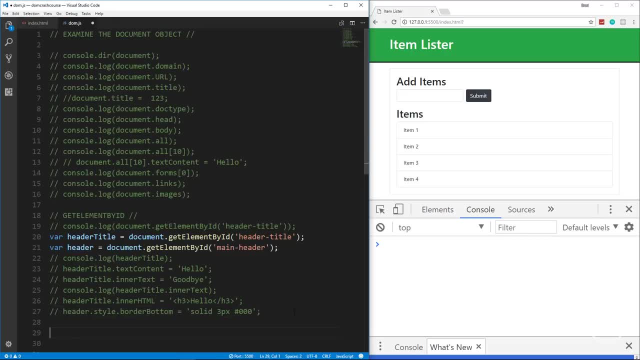 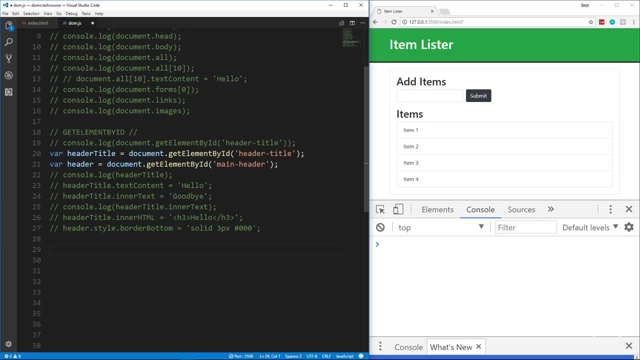 All right, So all stuff that used to be used with jQuery but should be used with vanilla JavaScript. Now you can see how easy it is, So next thing we're going to do is look at another thing. All right, So we're going to go to our selector. 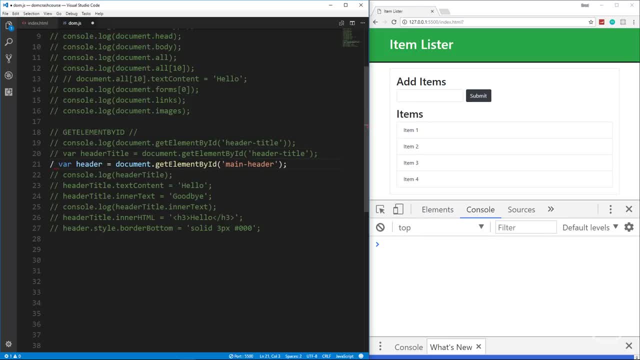 I'm going to comment these out too. So we're going to look at getting elements by class name. Okay, So let's say get elements by class name. Now notice that it's elements plural, So this works a little different. 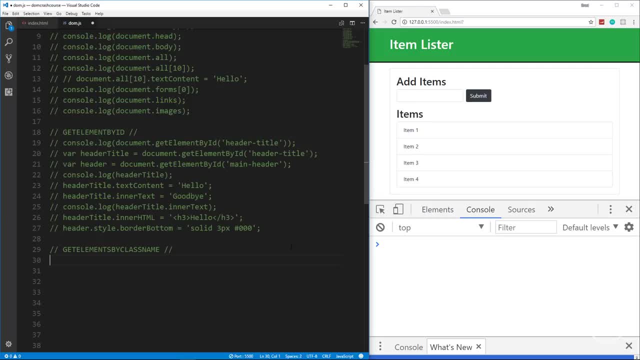 It's not like get element by class which doesn't actually exist. For that you would use query selector, but I'll get into that in a minute. So get elements by class name. Let's say we want to get All these list items. 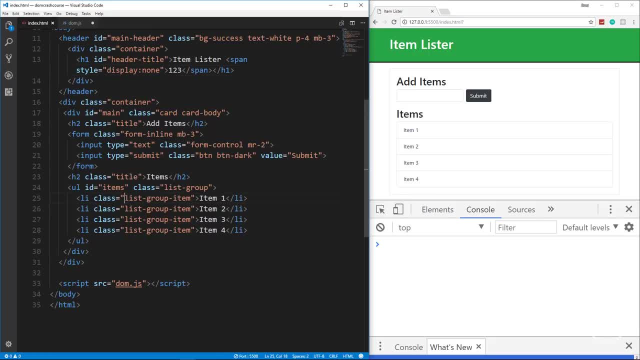 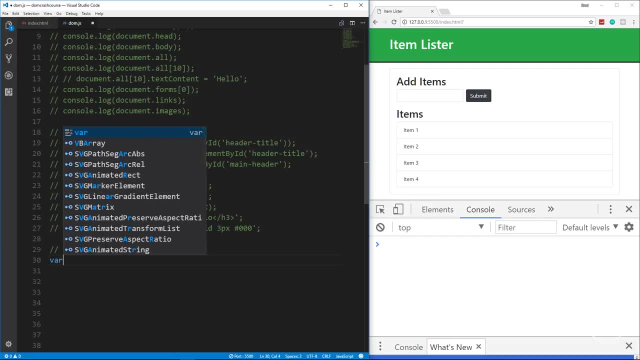 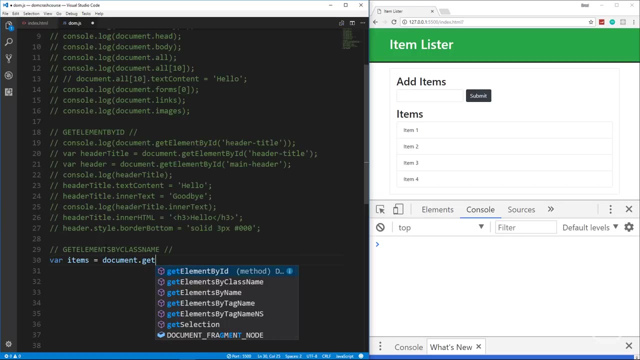 Okay, So we know that these list items have a class of list group item. So let's say we'll put it in a variable, So var items equals. and then we're going to say document dot, get. what am I doing? Get elements by class name and they have the class of list group. 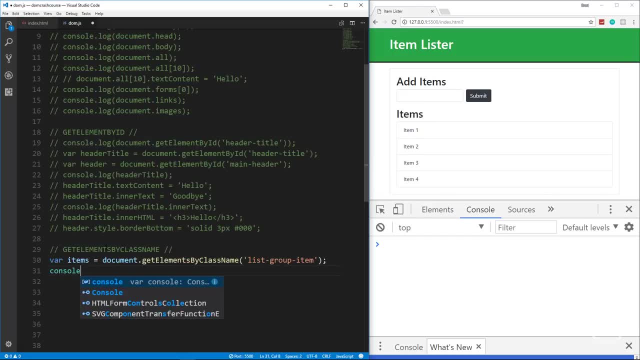 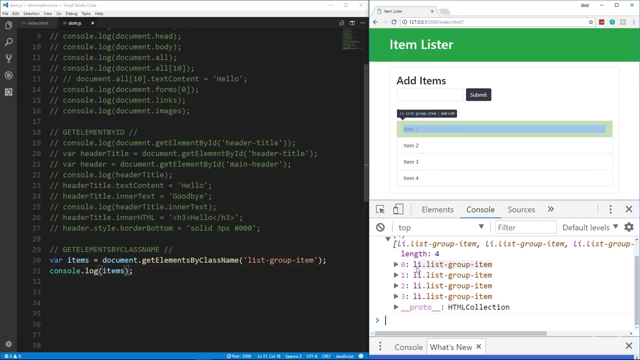 Items. Okay. So if we go ahead and we console dot log, Console dot log items, What do we get here? So what it gives us is an HTML collection. Okay, Just like document dot. all gives us, and each one has an index. 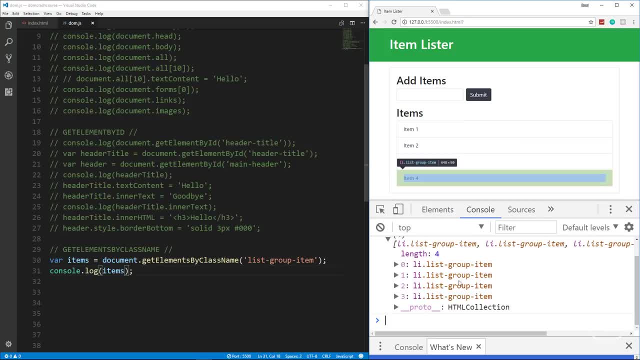 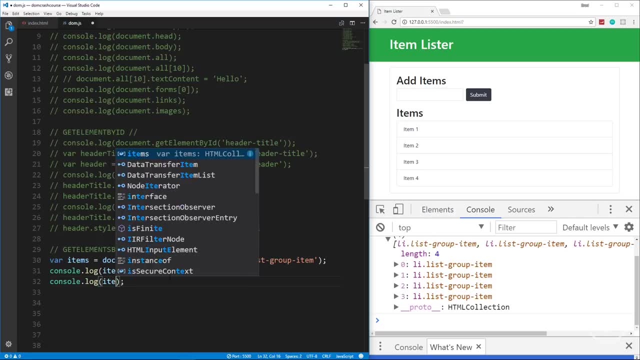 Okay, And you can see if I hover over one, it'll highlight in the in the browser. so we can access individual elements. Okay, So we can access individual elements. Okay, So we can access individual elements in the system by saying, like items, let's say we want the second one, we would use one because 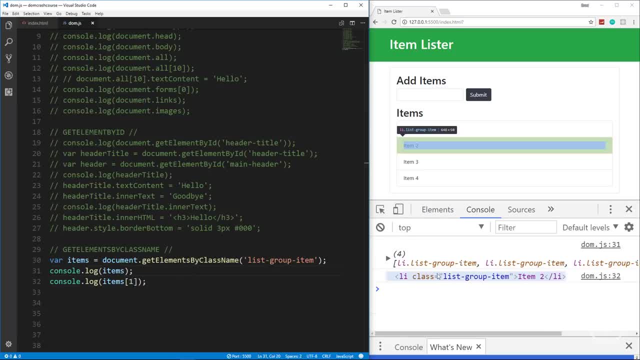 they're zero based. so we'll save and you'll see, it'll give us the item two. okay, that's in the one position. so if I wanted to, let's say, change the text of that, a particular item, I could say: items dot or not, items dot, but items one dot. 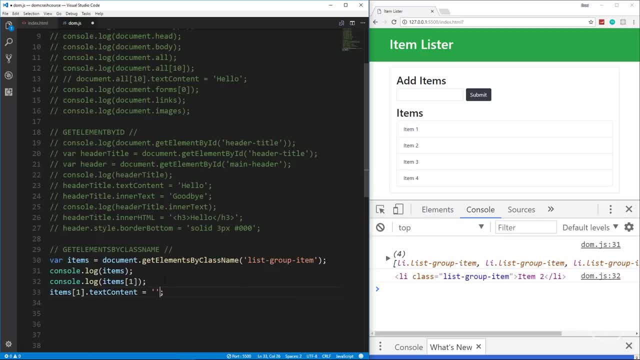 text content equals and we'll say hello to and save. and now you'll see that it actually says hello to. if I wanted to change the style, let's say items one dot, style dot, let's do font weight can't do that, we got to use camel case, so font. 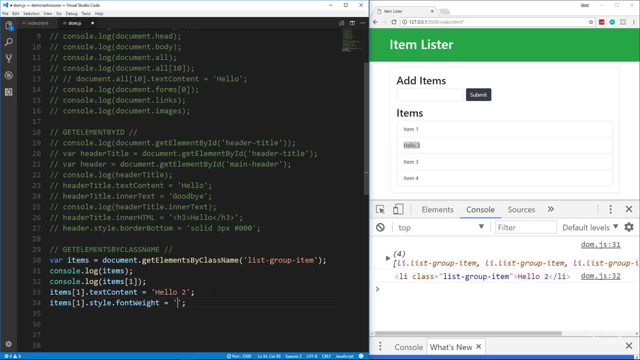 weight and we'll set that equal to you, bold and save. and now you can see that we've bolded that second one here. alright, if we wanted to do a background color for it, let's say items one, and will say style dot background color and we'll set it to, let's say, yellow and 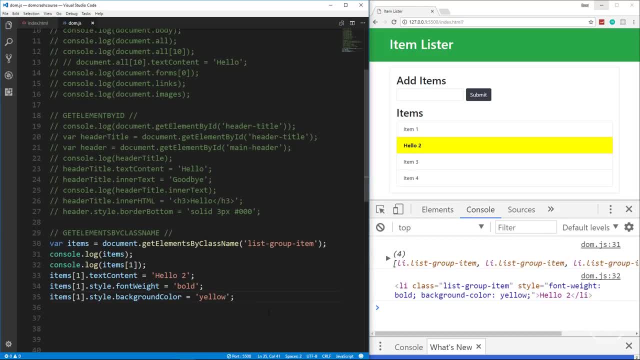 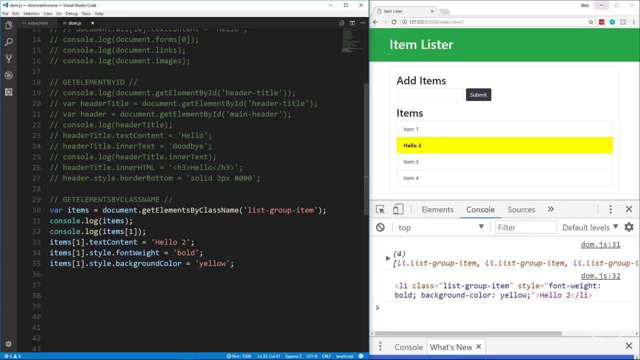 there we go ok. so you can see we can. we can do a lot, lot of the same stuff that we did we could do in jQuery. now where it gets tricky is if we want to add a style to all of these. so let's say, we want to give them all a light gray background. so if we 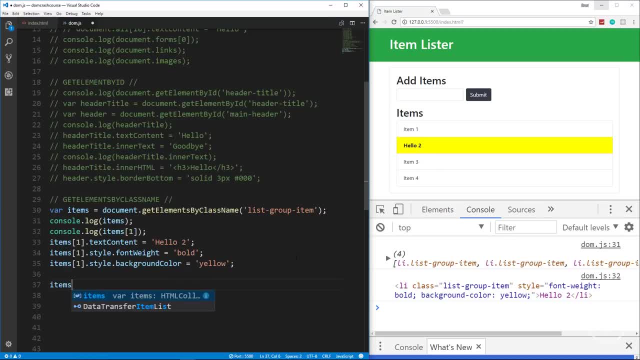 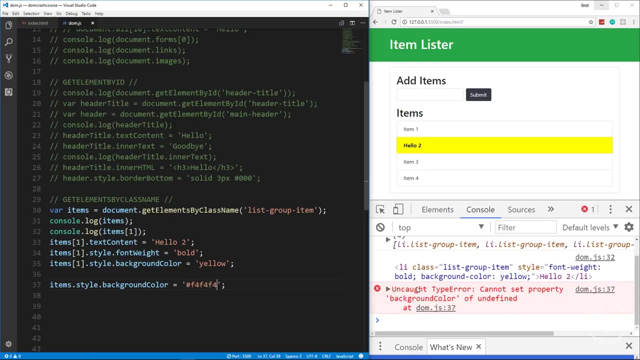 just say items, items, dot, style, dot, background color and set it to, let's say, light gray and save. that's not going to work. all right now. this isn't going to work because it's an, it's an HTML collection or it's an array. we have to actually loop through it to be able to do this. 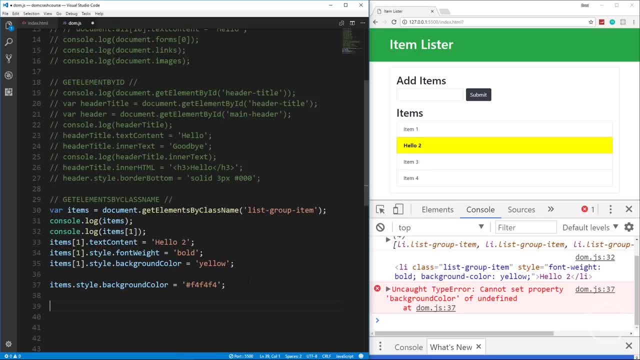 so what we can do is we can iterate through it with a for loop. so we're going to say for, we'll create a variable called i equals zero and we're going to say: as long as i is less than items dot length. okay, dot length is a property. it gets the, the number of items in that array. 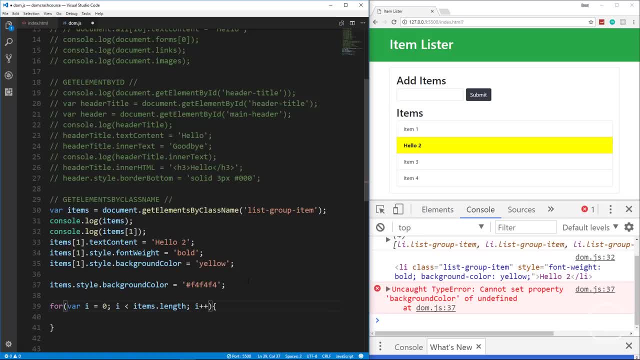 or collection, and then we just need to increment by one each time. and then here what we'll do is we'll say items and we want to get the current iteration, and then from there we can say: dot, style, dot- background color equals our gray color and save, oh, we need to. 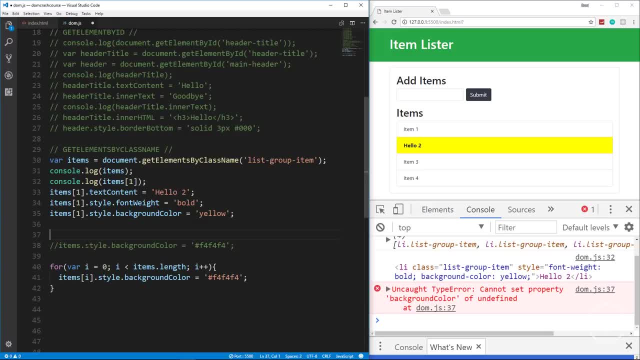 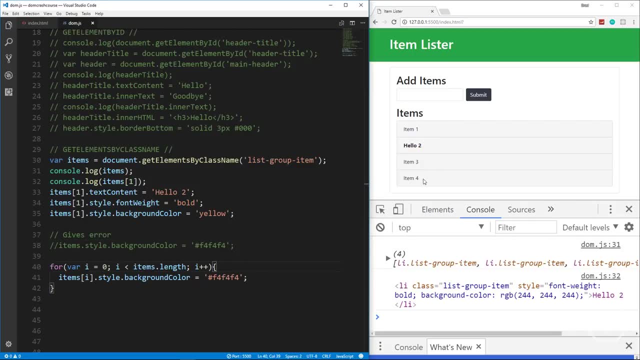 actually comment this out, because this is giving an error. actually, let's put a comment right here and we'll just say: gives error and save. and now you'll see that each one has a gray background. now, all right, so that is get elements by class name. now we're gonna take a look at get elements by tag name. now this: 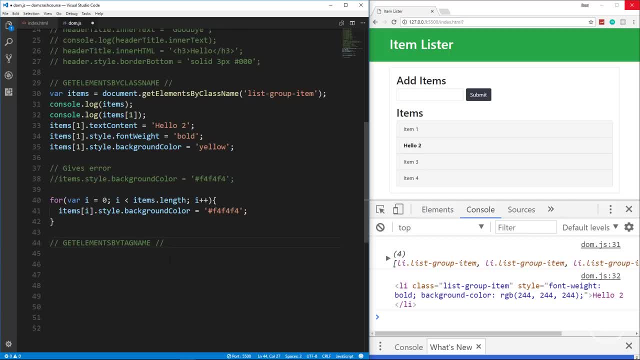 works basically the same way, except, instead of getting it by class, you're getting it by tag. so what I'm gonna do is I'm actually gonna copy this whole thing. I'm gonna copy it, and then I'm gonna comment it out. okay, we'll paste it. 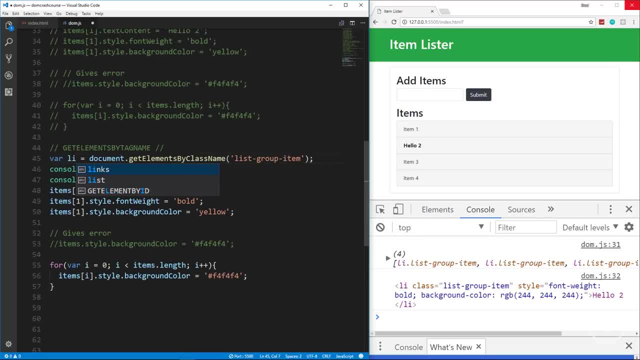 here, and then I'm gonna comment it out: okay, we'll paste it here, and then I'm gonna comment it out: okay, we'll paste it here. now let's change the variable to here. now, let's change the variable to here. now, let's change the variable to Li and what I want to do is say: get. 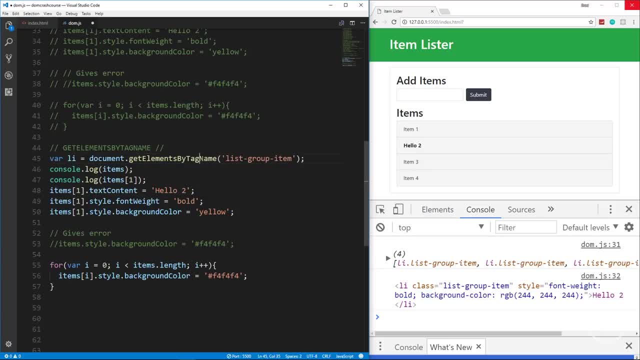 Li, and what I want to do is say: get Li. and what I want to do is say: get elements by tag name and then just pass elements by tag name and then just pass elements by tag name and then just pass in here Li. so it's gonna grab all the. 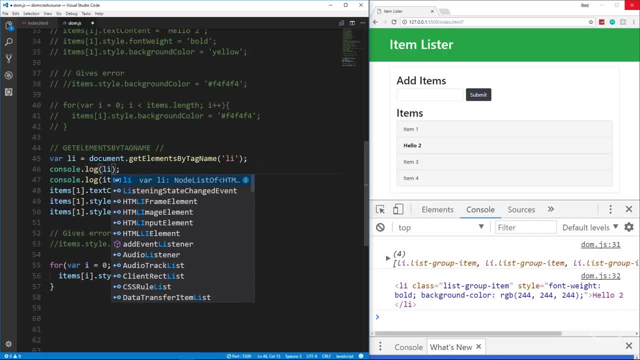 in here Li. so it's gonna grab all the in here Li. so it's gonna grab all the allies on the page, and then let's console allies on the page, and then let's console allies on the page, and then let's console log Li. we can get each Li by its. by its. 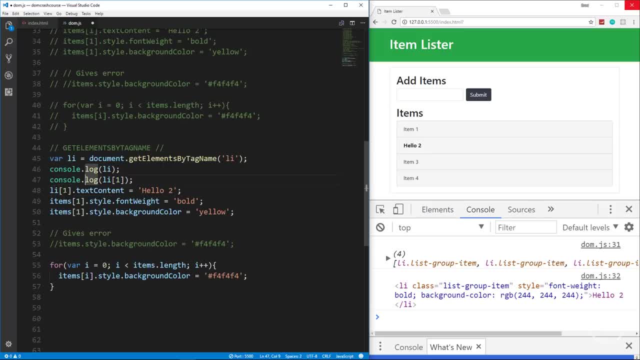 log Li. we can get each Li by its, by its log Li. we can get each Li by its, by its index. so let's change this to Li. so this index. so let's change this to Li, so this index. so let's change this to Li. so this should basically do the same exact thing. 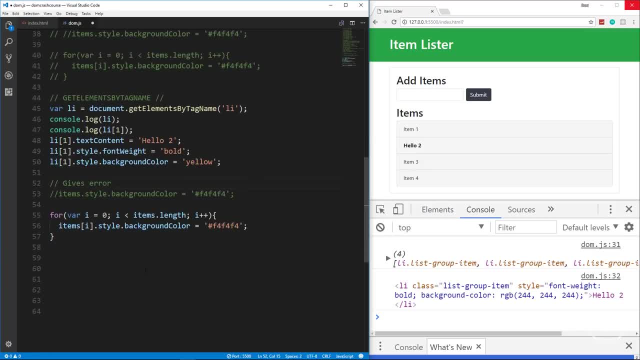 should basically do the same exact thing. should basically do the same exact thing. we're just not using the class we're. we're just not using the class we're. we're just not using the class. we're using the Li and then down here we can using the Li, and then down here we can. 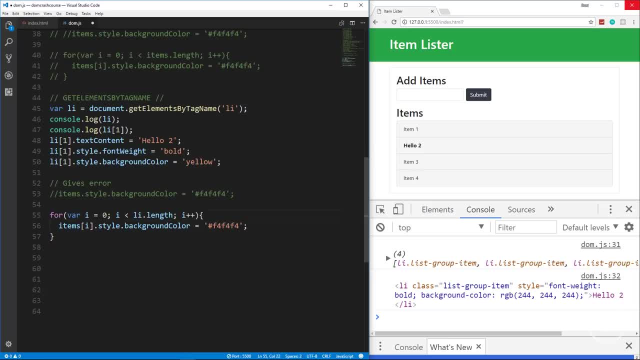 using the Li and then down here we can loop through. it works the same way. so Li loop through it works the same way. so Li loop through it works the same way. so Li. dot length save- let's save it and it. dot length save- let's save it and it. 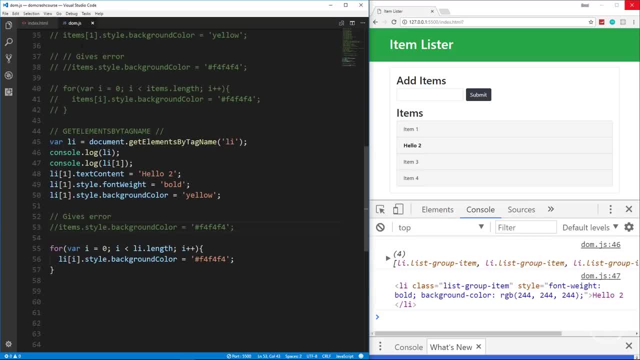 dot length: save, let's save it. and it does the same thing. all right now. if I does the same thing, all right now. if I does the same thing, all right now if I were to add another list item here, so were to add another list item here. so 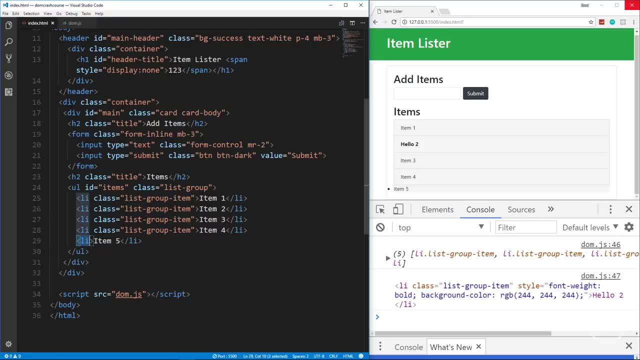 were to add another list item here. so class of list group item. it still class of list group item. it still class of list group item. it still applies because it's an Li. it's going by. applies because it's an Li. it's going by. applies because it's an Li. it's going by the tag, not by the class. if I were to 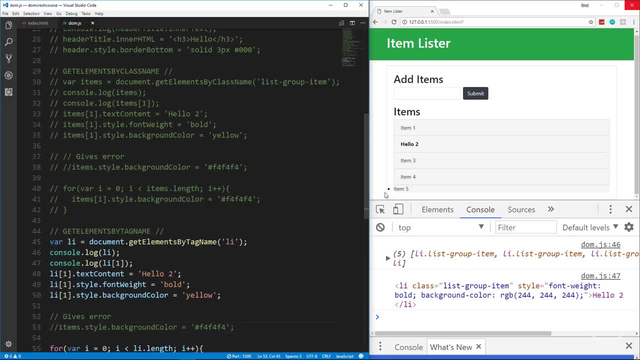 the tag, not by the class. if I were to the tag, not by the class, if I were to just do it by the class like I did up, just do it by the class, like I did up, just do it by the class like I did up here, then then that would have this. here, then then that would have this here, then then that would have. this would have no effect, all right, let me would have no effect. all right, let me would have no effect. all right, let me just show you what I mean. so if I just show you what I mean, so if I 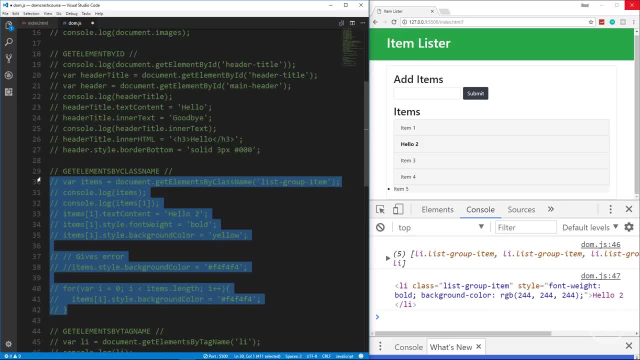 just show you what I mean. so if I comment that out and we uncomment this comment that out and we uncomment this comment that out and we uncomment this and save, you'll see that now that this and save, you'll see that now that this and save, you'll see that now that this stuff, nothing's being applied, this this, 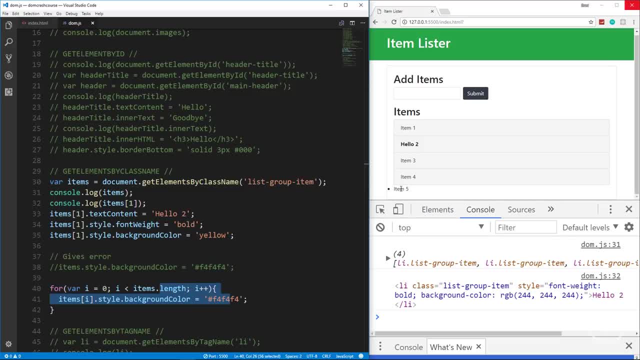 stuff- nothing's being applied. this, this stuff- nothing's being applied. this, this gray background, and all that is not gray background and all that is not gray background and all that is not applying to this because it doesn't have applying to this because it doesn't have. 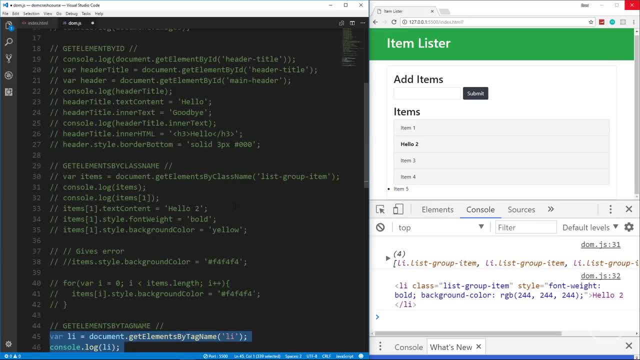 applying to this because it doesn't have that class, all right. so hopefully that that class all right. so hopefully that that class all right. so hopefully that makes sense all right. so let's get makes sense all right. so let's get makes sense all right. so let's get element by tags name. I'm not going to. 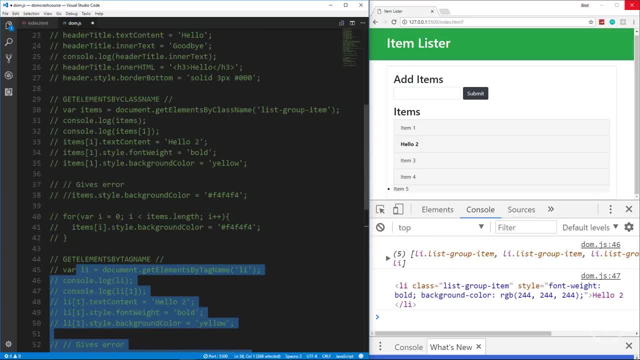 element by tags name. I'm not going to element by tags name. I'm not going to spend too much time on it. because it's spend too much time on it because it's spend too much time on it because it's identical to the class name. now what I 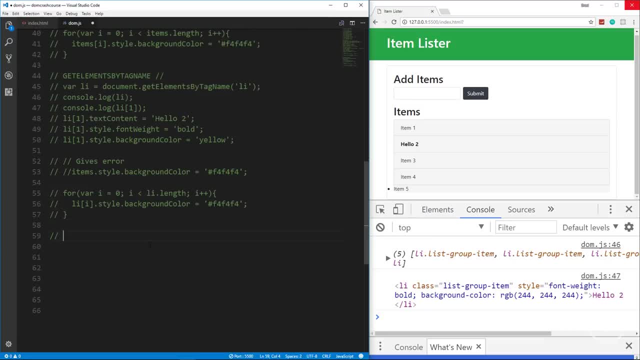 identical to the class name. now what I identical to the class name. now, what I want to do is look at query selector. want to do is look at query selector. want to do is look at query selector. alright, so this is an important one. so, alright, so this is an important one. so 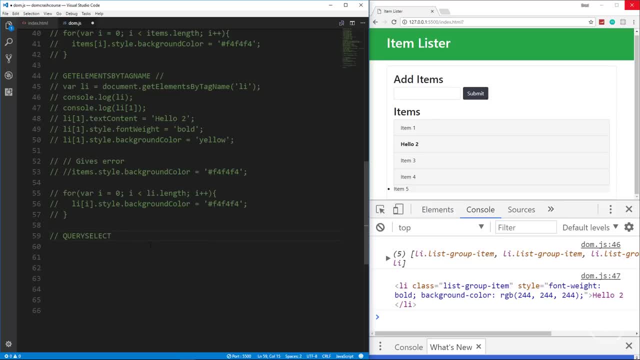 alright, so this is an important one, so query selector. so for this, this works. query selector. so for this, this works, query selector. so for this, this works pretty much just like jQuery. okay, the pretty much just like jQuery. okay, the pretty much just like jQuery. okay, the only big difference is: it's it only? 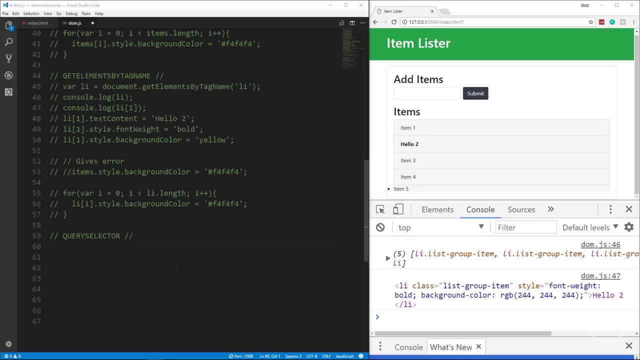 only big difference. is it's it only only big difference? is it's it only what you're all you use it only for one? what you're all you use it only for one. what you're all you use it only for one item. okay, if you want to use more than. 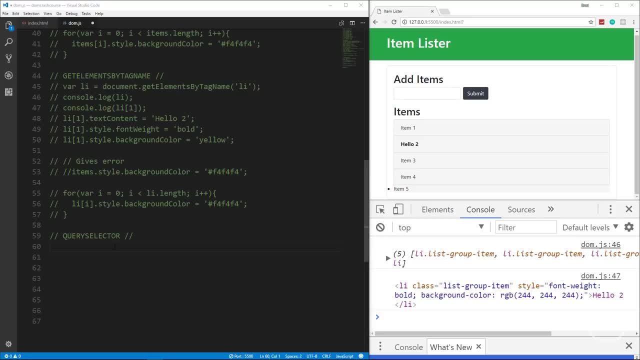 item. okay, if you want to use more than item. okay. if you want to use more than one item, then you're gonna use query. one item, then you're gonna use query one item, then you're gonna use query selector. all which I'm gonna go over in a 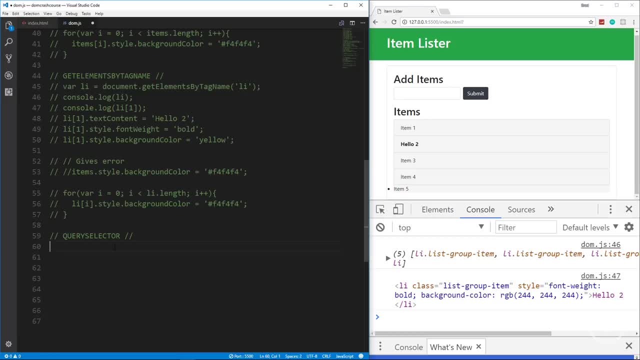 selector, all which I'm gonna go over in a selector, all which I'm gonna go over in a second as well, alright so, and it only second as well, alright so, and it only second as well, alright so, and it only affect it only grabs the first one. so if 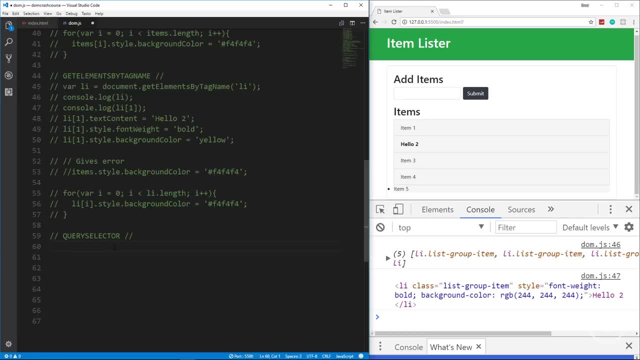 affect, it only grabs the first one. so if affect, it only grabs the first one. so if we try to grab, let's say the class of we try to grab, let's say the class of we try to grab, let's say the class of title, and there's more than one title on. 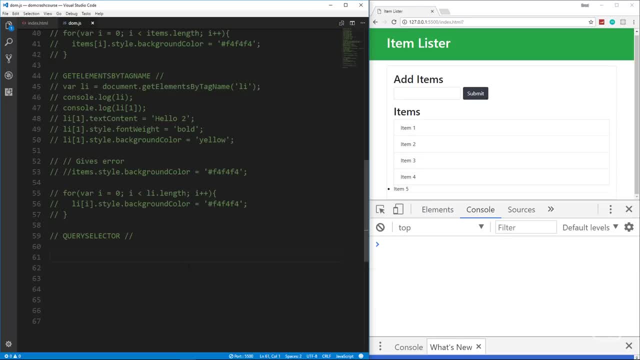 title and there's more than one title on title and there's more than one title on the page, it's gonna grab the first one. the page. it's gonna grab the first one. the page, it's gonna grab the first one. so let's go ahead and save this and 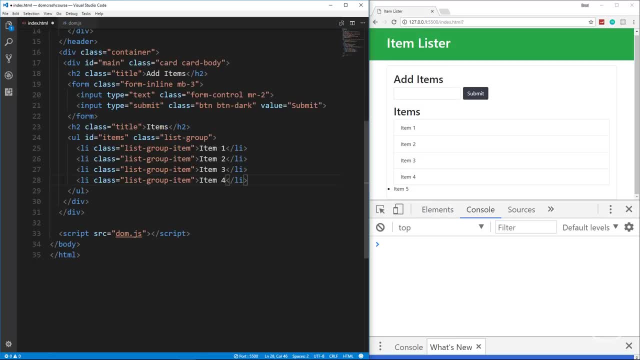 so let's go ahead and save this. and so let's go ahead and save this and let's get rid of that extra Li. we added. let's get rid of that extra Li. we added. let's get rid of that extra Li. we added. alright, so we'll save that and we're 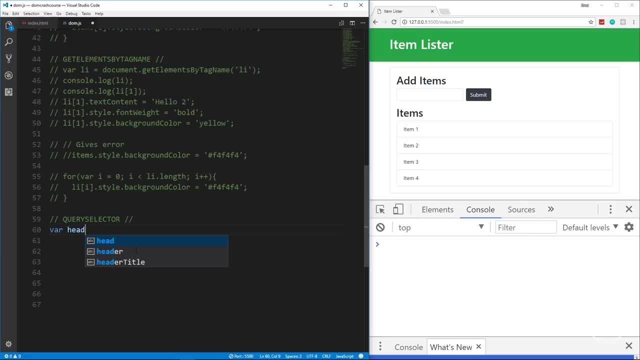 alright, so we'll save that. and we're alright, so we'll save that. and we're gonna say let's save our header. and gonna say let's save our header. and gonna say let's save our header and we're gonna say: document dot query. we're gonna say document dot query. 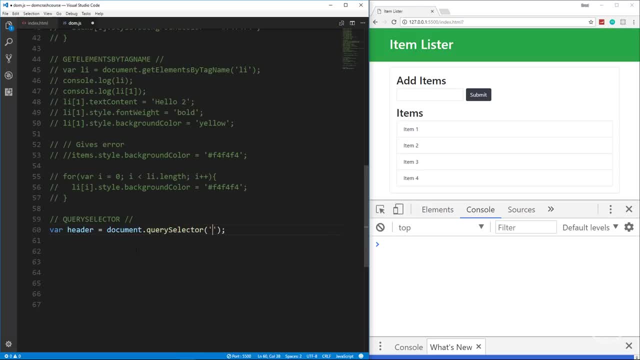 we're gonna say: document dot, query selector and we can use anything we want selector and we can use anything we want selector and we can use anything we want in here, so we can use tags. you could in here, so we can use tags. you could in here, so we can use tags. you could grab a list item. you could grab a class. 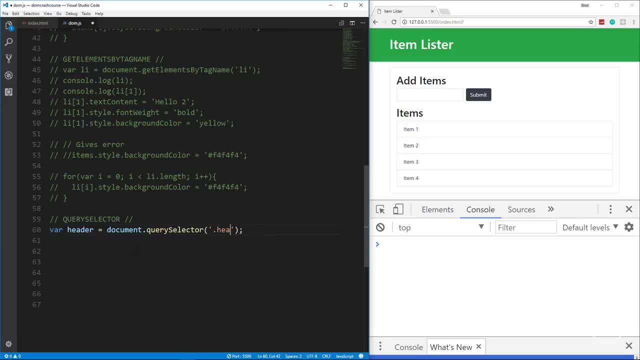 grab a list item, you could grab a class. grab a list item, you could grab a class. okay, so you could say dot header you. okay, so you could say dot header you. okay, so you could say dot header. you can use any CSS selector just like you can use any CSS selector, just like you. 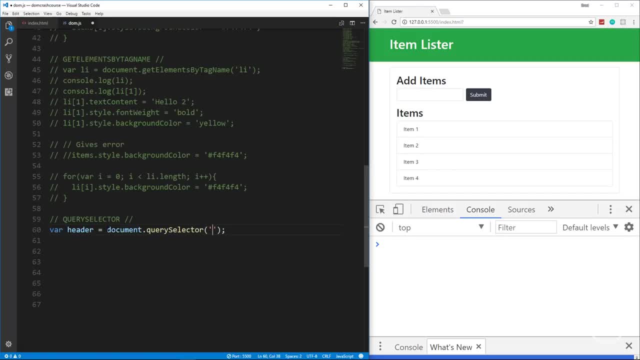 can use any CSS selector, just like you could with jQuery. okay, so just replace could with jQuery. okay, so just replace could with jQuery. okay, so just replace the jQuery money sign, like that, with the jQuery money sign, like that, with the jQuery money sign, like that with documents, document dot query selector. so 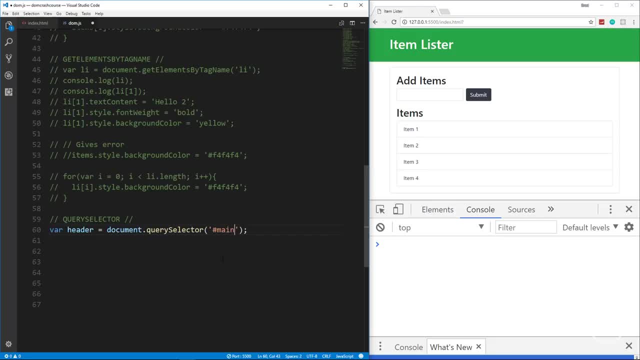 documents document, dot. query selector. so documents- document, dot. query selector. so if we want to grab the header, for, if we want to grab the header, for, if we want to grab the header, for instance, it has an ID of main header. so, instance, it has an ID of main header. so 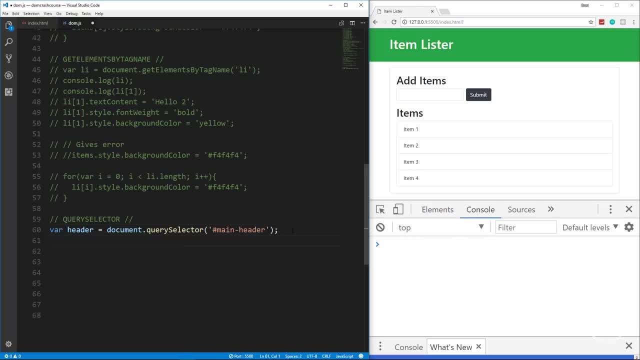 instance, it has an ID of main header. so make sure you use that hash right there. make sure you use that hash right there. make sure you use that hash right there, all right. and then we could say: header all right. and then we could say: header all right. and then we could say: header: dot. style dot: border bottom. we'll set it. 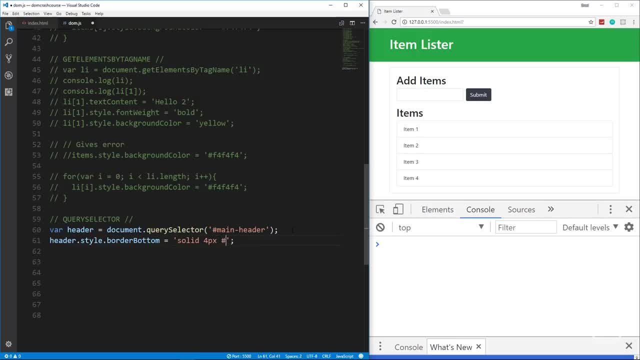 dot style dot border bottom. we'll set it. dot style dot border bottom. we'll set it to solid four pixels and gray save and to solid four pixels and gray save and to solid four pixels and gray save. and now you can see it has that, that border. 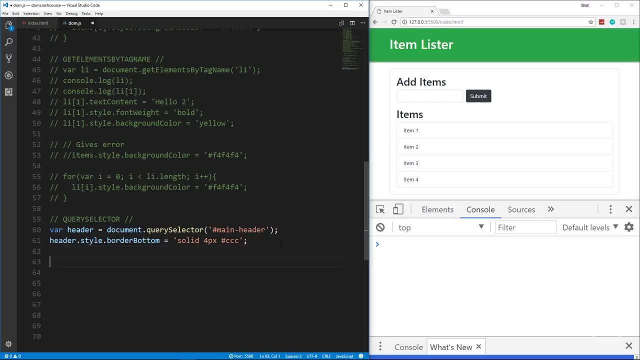 now you can see it has that that border. now you can see it has that that border, all right. so another thing we could all right, so another thing we could all right. so another thing we could select is: let's grab the input we haven't. select, is: let's grab the input we haven't. 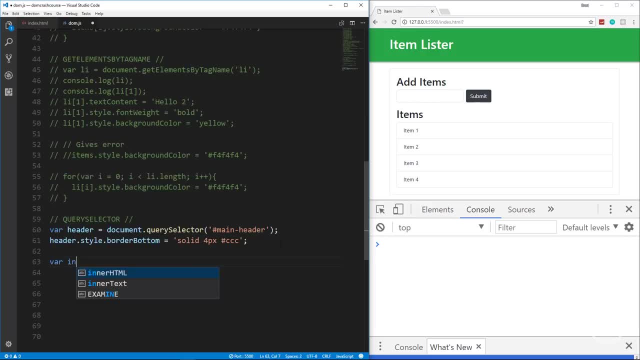 select is: let's grab the input. we haven't done anything with that input form, so done anything with that input form, so done anything with that input form. so let's say var input and let's set this. let's say var input and let's set this. 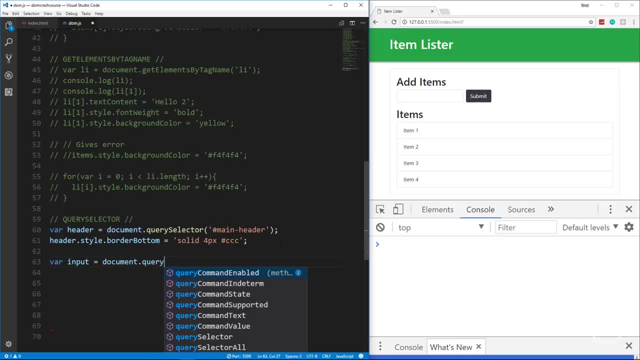 let's say var input and let's set this to document dot query selector and we to document dot query selector and we to document dot query selector, and we want to grab the input and we'll say want to grab the input and we'll say want to grab the input and we'll say input, dot value equals hello world and 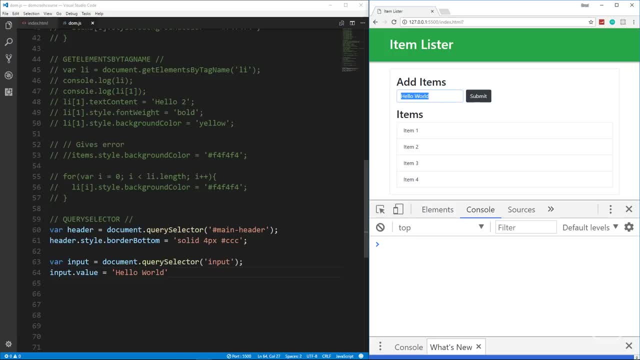 input dot value equals hello world. and input dot value equals hello world and save. and you can see now we've actually save. and you can see now we've actually save. and you can see now we've actually added a value to that input now even. added a value to that input now even. 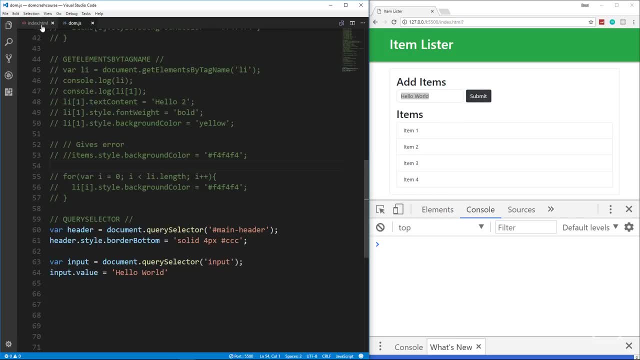 added a value to that input. now, even though there's two inputs on the page, though there's two inputs on the page, though there's two inputs on the page, because this, this button, this is actually because this, this button, this is actually because this, this button, this is actually an input as well. it only grabbed the. 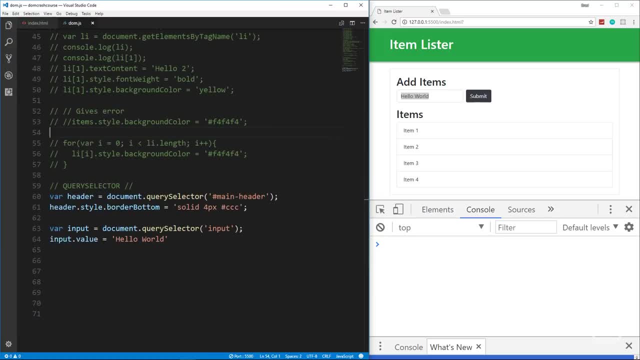 an input as well. it only grabbed the an input as well. it only grabbed the first one. okay, so it's gonna grab the first one. okay, so it's gonna grab the first one. okay, so it's gonna grab the first one by default now with query. first one by default now with query. 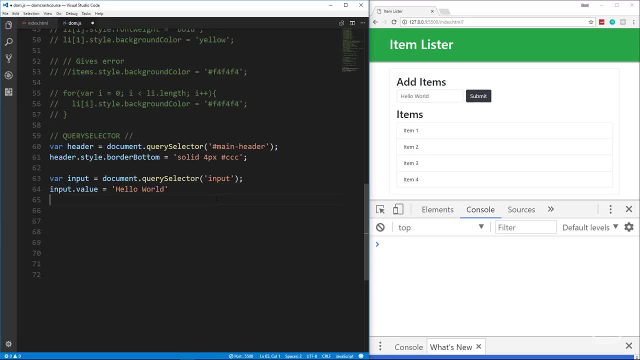 first one by default. now, with query selector, we can use any CSS selector, so selector, we can use any CSS selector, so selector, we can use any CSS selector. so what I'm gonna do now is I'm gonna say: what I'm gonna do now is I'm gonna say: 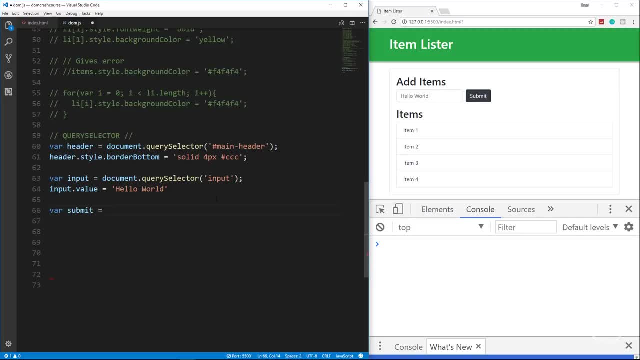 what I'm gonna do now is I'm gonna say var submit and let's set this to var submit and let's set this to var submit. and let's set this to document dot query selector and instead document dot query selector and instead document dot query selector. and instead of just input, let's use the input and 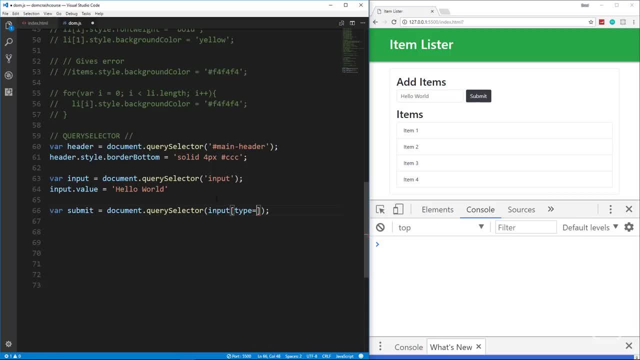 of just input, let's use the input. and of just input, let's use the input. and then brackets, and we can say the type, then brackets, and we can say the type, then brackets, and we can say the type: equals- submit. okay, just like we could do. equals- submit. okay, just like we could do. 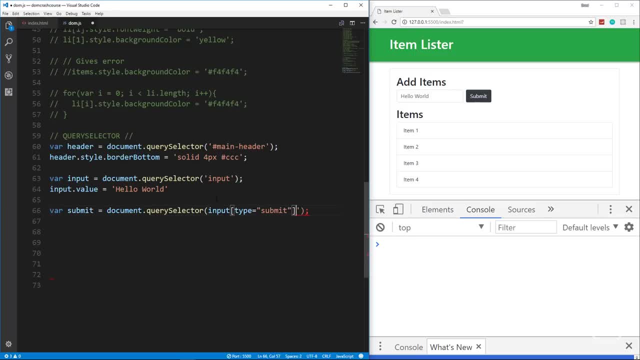 equals submit. okay, just like we could do in CSS. this should actually be in quotes in CSS. this should actually be in quotes in CSS. this should actually be in quotes, though. alright, so if we do that. and then though, alright, so if we do that. and then though, alright, so if we do that, and then we say submit dot value, and let's see. 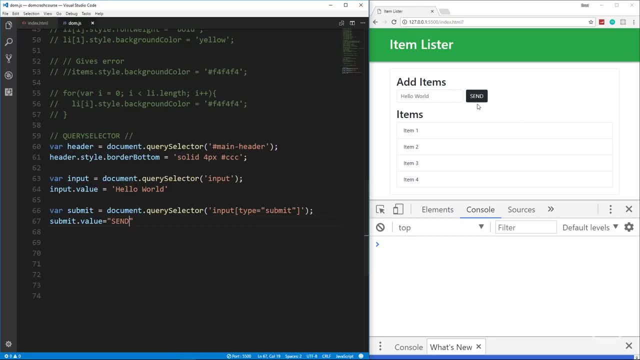 we say submit dot value. and let's see, we say submit dot value. and let's see, we'll still change it to send and save. we'll still change it to send and save. we'll still change it to send and save. and now you can see, you've actually 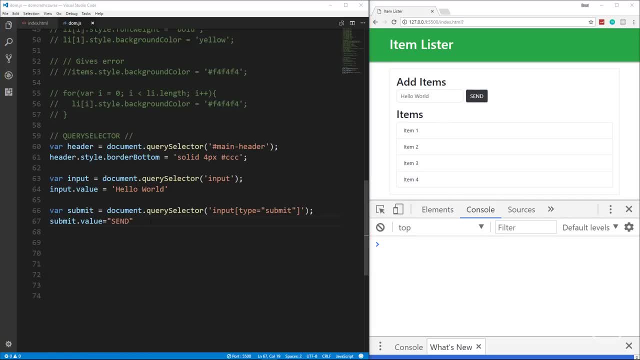 and now you can see you've actually- and now you can see you've actually- changed the button to send all right. so changed the button to send all right, so changed the button to send all right. so what about these list items? what if we? what about these list items? what if we? 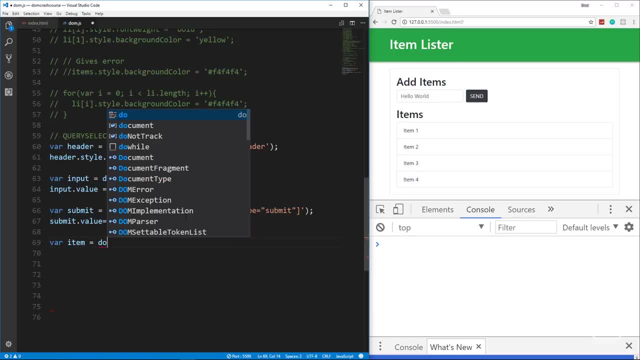 what about these list items? what if we were to say var item and send it. set it were to say var item and send it set it were to say var item and send it? set it to document dot query selector and we to document dot query selector and we. 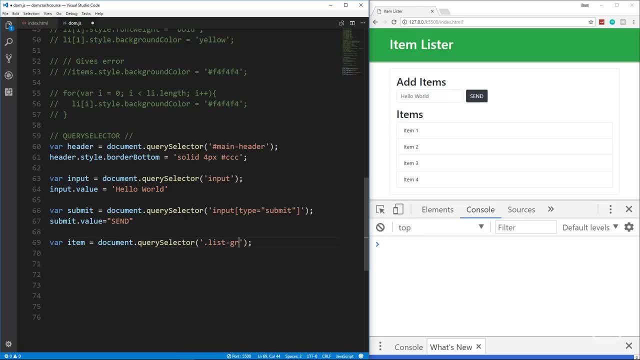 to document dot query selector and we put in here a class of list. what is it put in here? a class of list? what is it put in here? a class of list, what is it list group item: all right, and then let's list. group item: all right, and then let's. 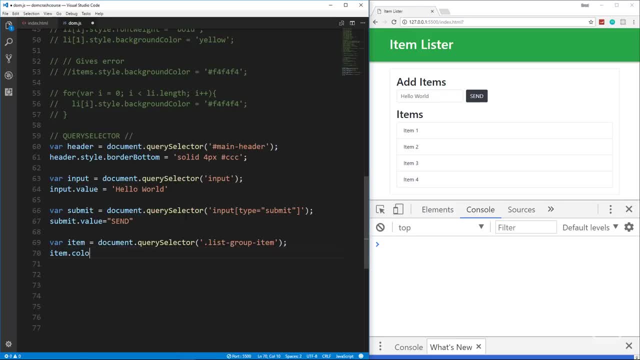 list group item. all right. and then let's say item dot color, not color item dot. say item dot color, not color item dot. say item dot color, not color item dot. style dot color equals red. what happens? style dot color equals red. what happens? style dot color equals red. what happens? it's gonna get the first one on the page. 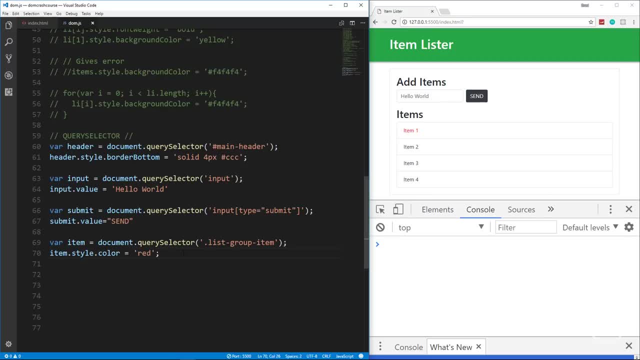 it's gonna get the first one on the page. it's gonna get the first one on the page. all right now. let's say we wanted to get all right now. let's say we wanted to get all right now. let's say we wanted to get the last one. we could use the the seat. 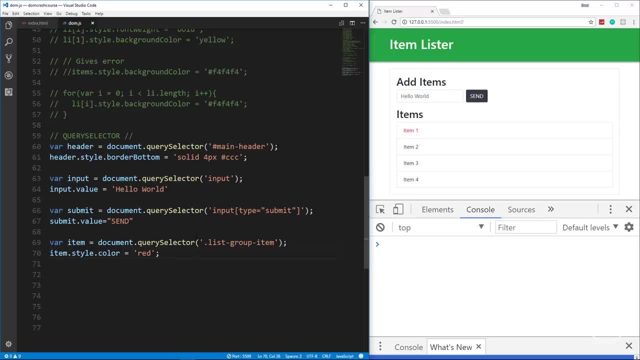 the last one. we could use the the seat, the last one. we could use the the seat, the CSS, last child. okay, so we'll say var, the CSS, last child. okay, so we'll say var, the CSS last child. okay, so we'll say var and let's say last item. actually I'll 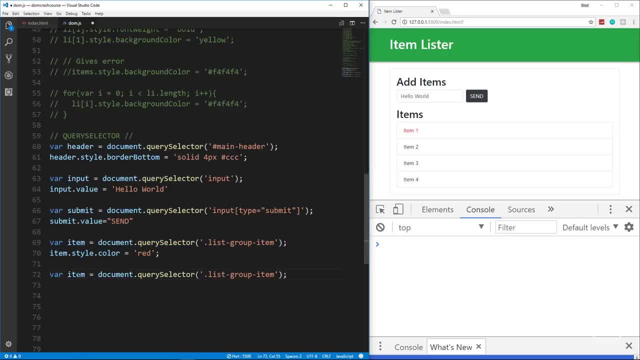 and let's say last item. actually I'll. and let's say last item, actually I'll just copy this, so we'll say last item. just copy this, so we'll say last item. just copy this, so we'll say last item and we'll select list: group, item, colon. 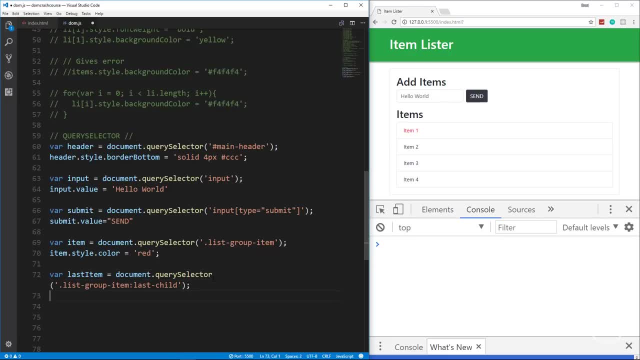 and we'll select list group item colon and we'll select list group item colon. and then let's say last item dot style and then let's say last item dot style and then let's say last item dot style. dot color equals blue and save, and dot color equals blue and save, and. 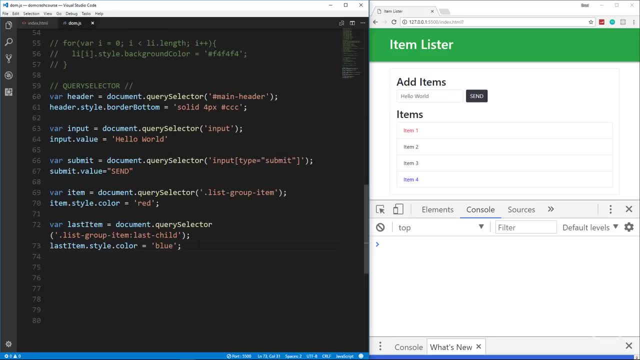 dot color equals blue and save. and you'll see that now the last one is blue. you'll see that now the last one is blue. you'll see that now the last one is blue. all right, we could also use our nth. all right, we could also use our nth. 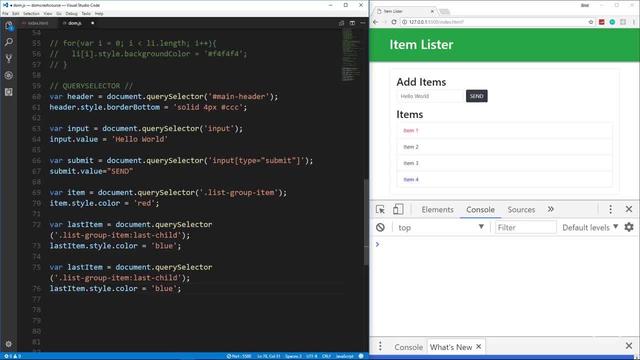 all right, we could also use our nth child. so let's say we want to grab the child. so let's say we want to grab the child. so let's say we want to grab the second one. so we'll say second item and second one. so we'll say second item and. 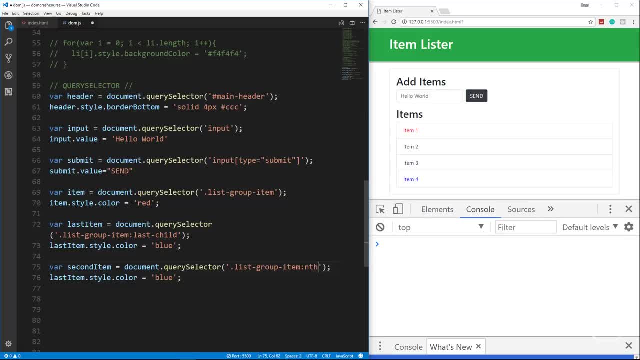 second one. so we'll say second item and we'll change this to: let's say: we'll change this to: let's say we'll change this to: let's say nth child 2, and then we'll change this to nth child 2, and then we'll change this to: 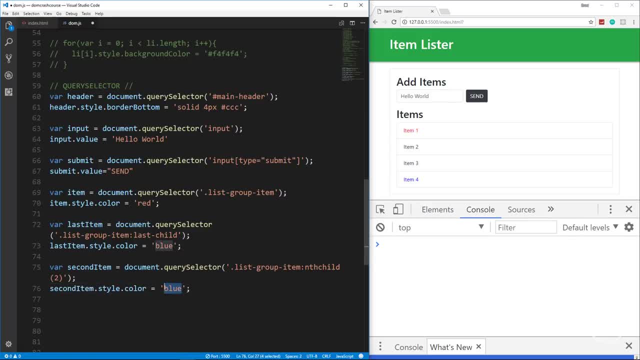 nth child 2, and then we'll change this to second item and we'll change it to second item and we'll change it to second item and we'll change it to: let's say, I don't know coral and save. let's say, I don't know coral and save. 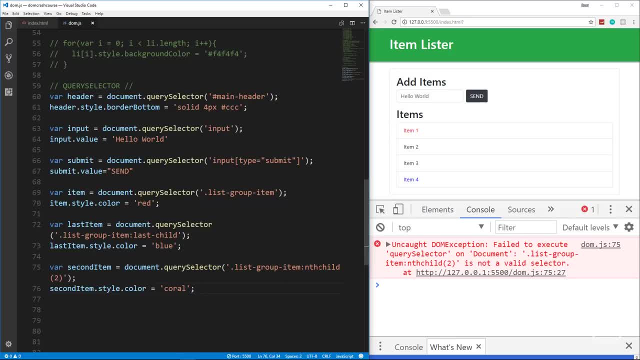 let's say, I don't know coral and save. wait a minute and look at the dash there. wait a minute and look at the dash there. wait a minute and look at the dash- there we go. so now the second one is coral- we go. so now the second one is coral. 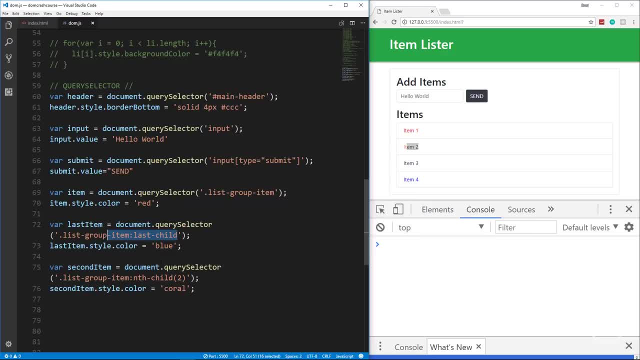 we go. so now the second one is coral. okay, so we can use these CSS pseudo. okay, so we can use these CSS pseudo. okay, so we can use these CSS pseudo classes or pseudo selectors, whatever classes, or pseudo selectors, whatever classes, or pseudo selectors, whatever they're called. all right, so what about? 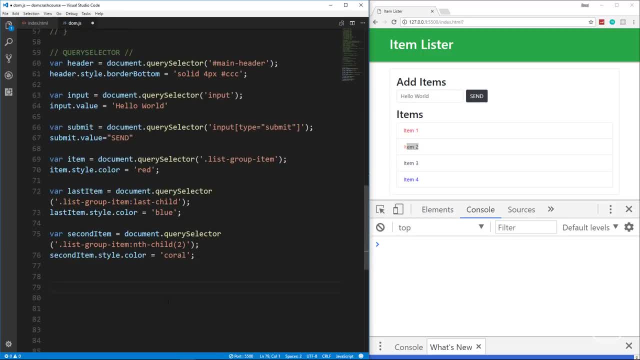 they're called all right. so what about? they're called all right. so what about query selector all? let's take a look at query selector all. let's take a look at query selector all. let's take a look at that. so query selector- all works similar. that, so query selector- all works similar. 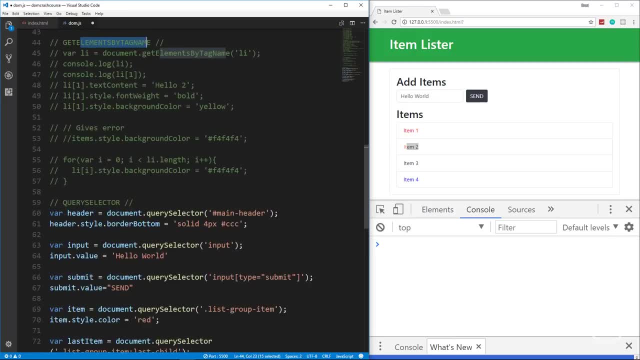 that. so query selector all works similar to like: get elements by tag name. get to like: get elements by tag name. get to like: get elements by tag name, get elements by class name. it's gonna grab elements by class name. it's gonna grab elements by class name. it's gonna grab more than one thing. so what I'm gonna do? 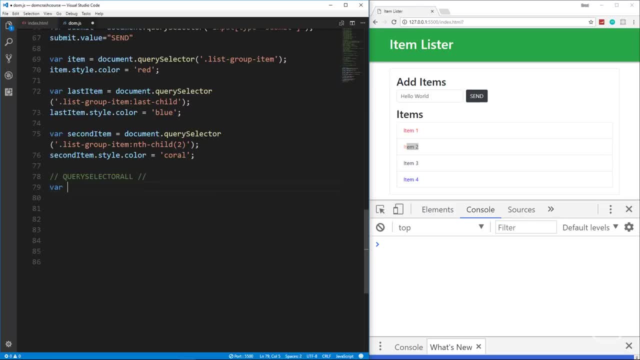 more than one thing. so what I'm gonna do more than one thing. so what I'm gonna do here is create a variable. here is create a variable. here is create a variable. let's see, I think we have two title. let's see, I think we have two title. 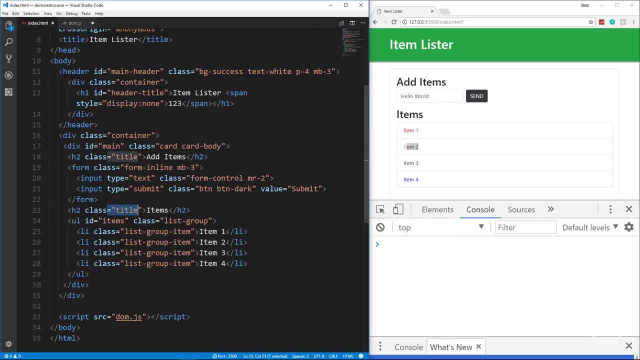 let's see, I think we have two title classes- yeah, we have h2 class title and classes- yeah, we have h2 class title and classes. yeah, we have h2 class title and h2 class title here, so let's grab both. h2 class title here, so let's grab both. 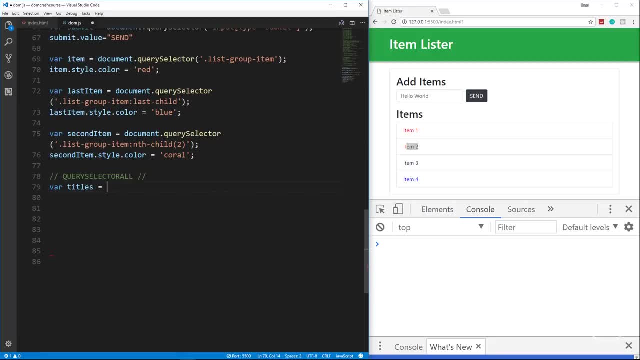 h2 class title here. so let's grab both of those. so we'll say titles equals of those. so we'll say titles equals of those. so we'll say titles equals document dot query selector all. and we document dot query selector all. and we document dot query selector all. and we want to get and we can put anything in. 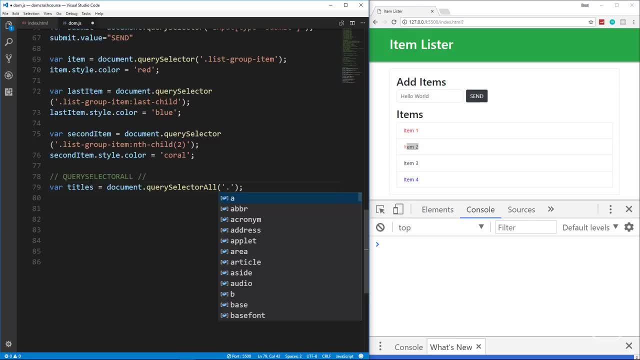 want to get and we can put anything in: want to get and we can put anything in here. classes IDs just tags anything. so here, classes IDs, just tags anything. so here, classes IDs, just tags anything. so we're gonna say class title: all right. we're gonna say class title all right. 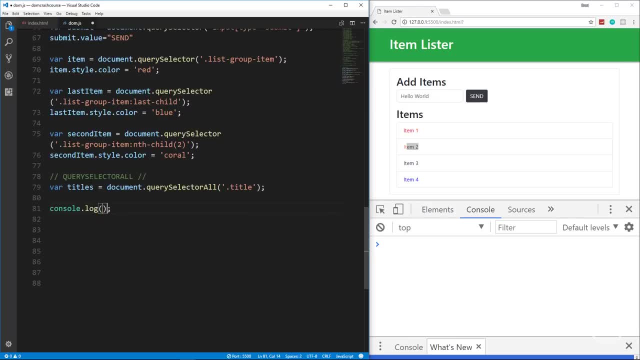 we're gonna say: class title: all right, and then let's go ahead and console dot. and then let's go ahead and console dot, and then let's go ahead and console dot. log titles- all right, I'm just gonna log titles. all right, I'm just gonna. 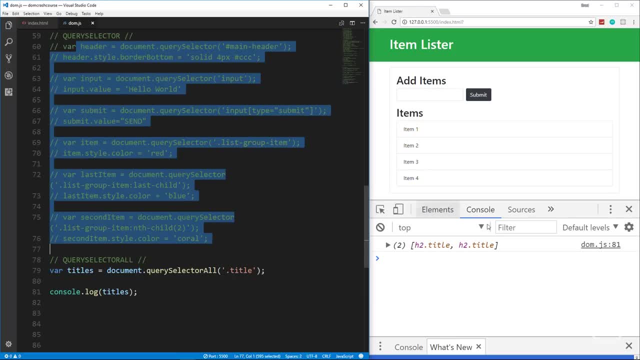 log titles. all right, I'm just gonna comment all this stuff out. okay, so that comment all this stuff out. okay, so that comment all this stuff out. okay, so that gives us what's called a node list, which gives us what's called a node list. which gives us what's called a node list, which is similar to a collection, except we can. 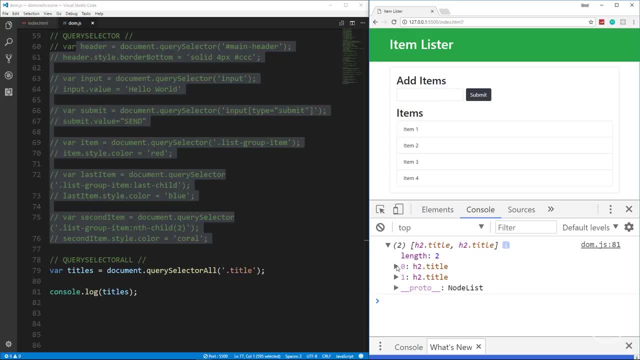 is similar to a collection, except we can is similar to a collection, except we can actually run array functions on a node. actually run array functions on a node, actually run array functions on a node list. so zero is going to be the first list, so zero is going to be the first. 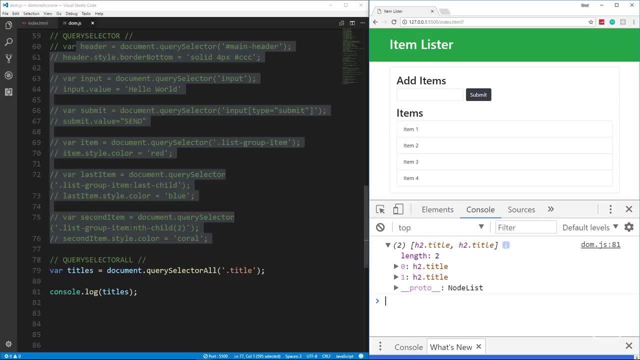 list. so zero is going to be the first title, which is that add items, and then title which is that add items, and then title which is that add items, and then one is the items, and of course we can. one is the items, and of course we can. 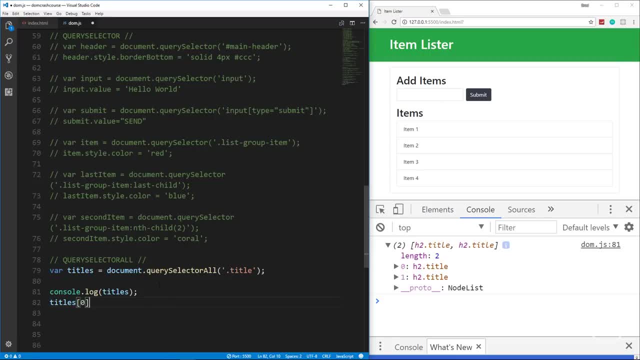 one is the items and of course we can access these like this. we could say: access these. like this. we could say: access these like this: we could say: titles: zero dot text content equals titles. zero dot text content equals titles. zero dot text content equals hello. and we'll save, and we'll change it. 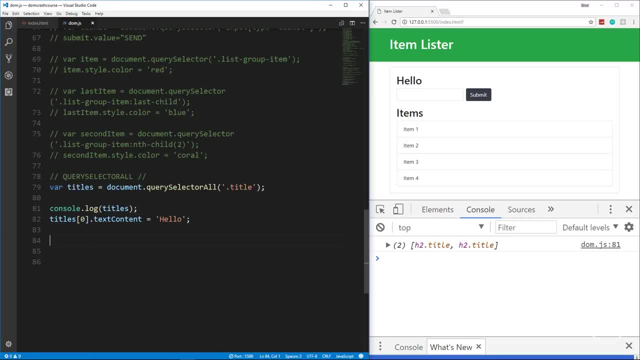 hello and we'll save. and we'll change it: hello and we'll save, and we'll change it that way. all right now. another thing that way, all right now. another thing that way, all right now. another thing that used to be really hard to do with. that used to be really hard to do with. 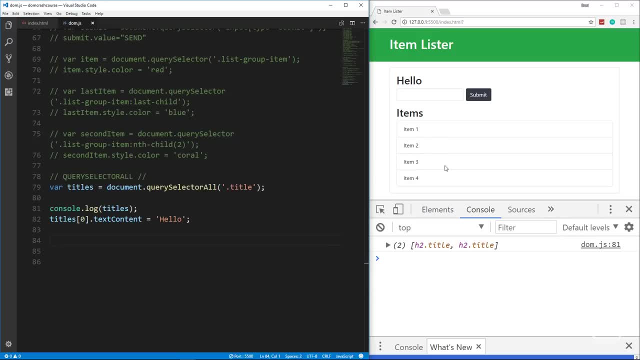 that used to be really hard to do with vanilla javascript would be to let's vanilla javascript would be to let's vanilla javascript would be to, let's say, alternate. let's say we want each say alternate. let's say we want each say alternate. let's say we want each other one to be gray, to have a gray. 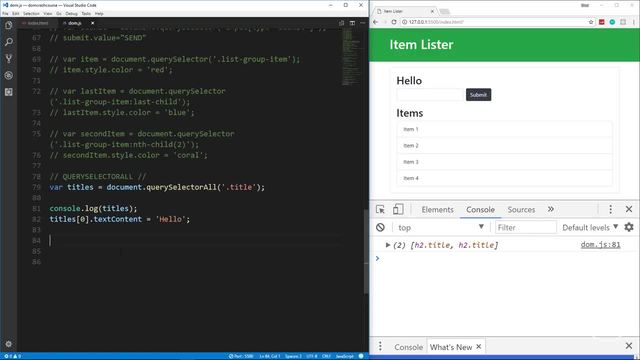 other one to be gray to have a gray, other one to be gray to have a gray background. but we can do that with query background, but we can do that with query background, but we can do that with query selector. all so what we'll do is we'll. 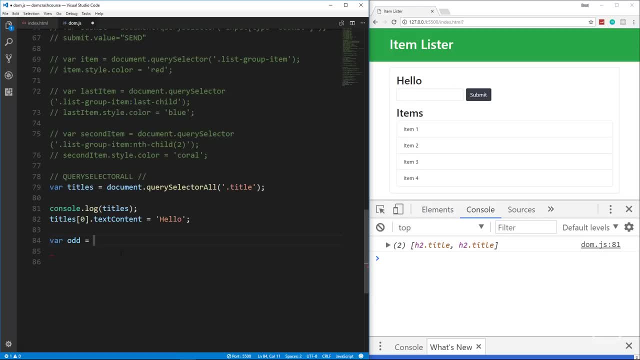 selector, all so. what we'll do is we'll selector, all so. what we'll do is we'll create a variable called odd, all right. create a variable called odd, all right. create a variable called odd, all right, and we'll set it to document dot query. and we'll set it to document dot query. 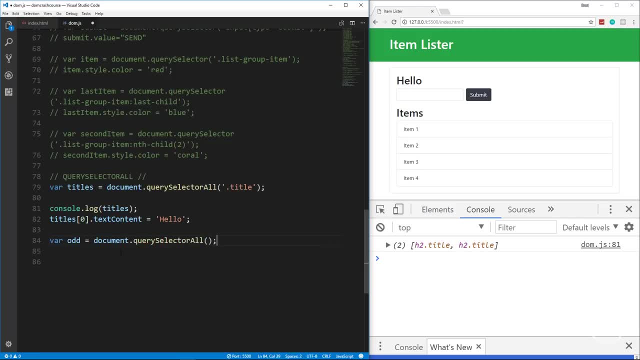 and we'll set it to document dot query: selector all, selector all, selector all. and we're going to use the and we're going to use the and we're going to use the. we're going to say li, we're going to say li, we're going to say li and let's use nth child. 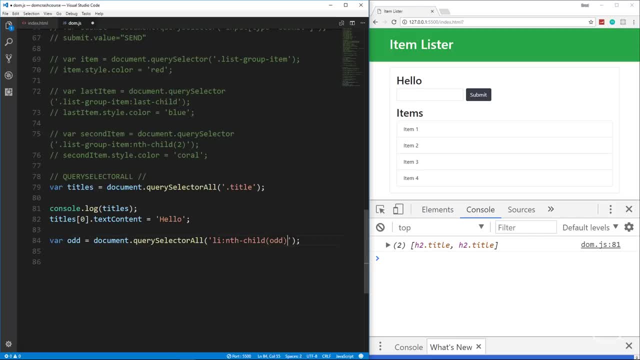 and let's use nth child. and let's use nth child and we'll pass in here: odd, okay now. and we'll pass in here: odd, okay now. and we'll pass in here: odd, okay now. this is a css selector. this is a pseudo. this is a css selector. this is a pseudo. 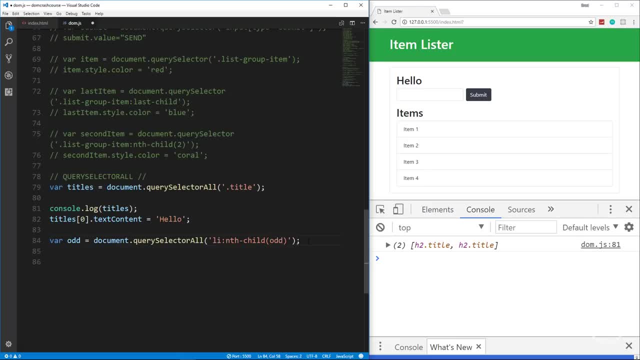 this is a css selector. this is a pseudo selector, selector, selector. so we're grabbing all the odd ones. and so we're grabbing all the odd ones. and so we're grabbing all the odd ones. and then what we'll do is we'll loop through. then what we'll do is we'll loop through. 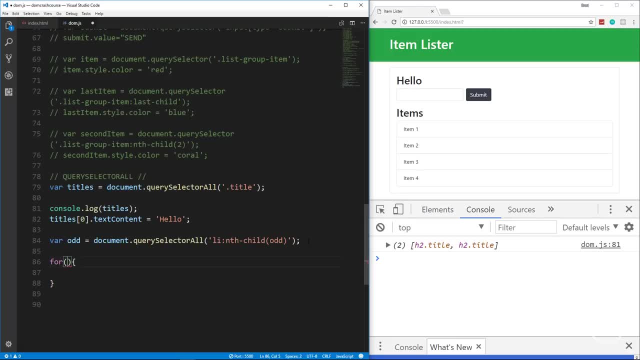 then what we'll do is: we'll loop through, we'll use a for loop, we'll use a for loop, we'll use a for loop, and we'll say for var, and we'll say for var, and we'll say for var. i equals zero as long as i is less than. 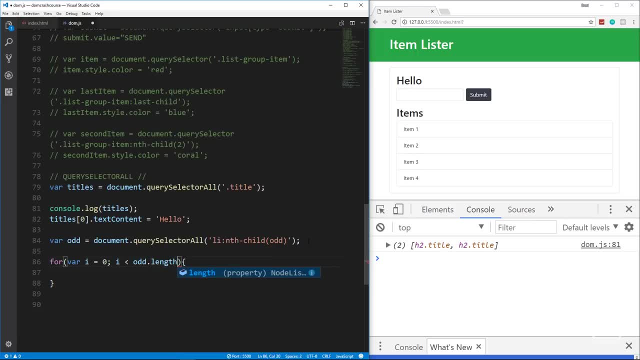 i equals zero as long as i is less than i equals zero as long as i is less than odd dot length, odd dot length, odd dot length. and let's see, we just want to increment, and let's see, we just want to increment, and let's see, we just want to increment by one. 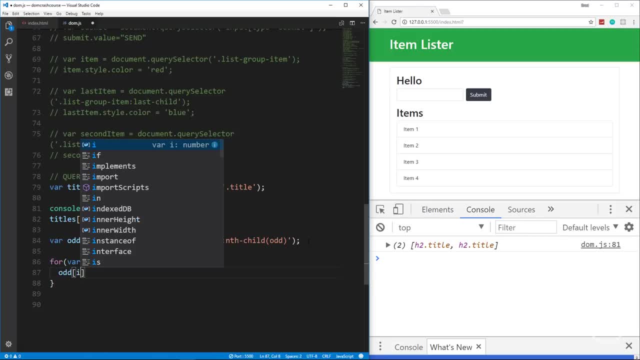 by one, by one, and then down here, what we'll do is we'll. and then, down here, what we'll do is we'll. and then down here, what we'll do is we'll say odd, say odd, say odd. we'll take the current iteration and we'll. 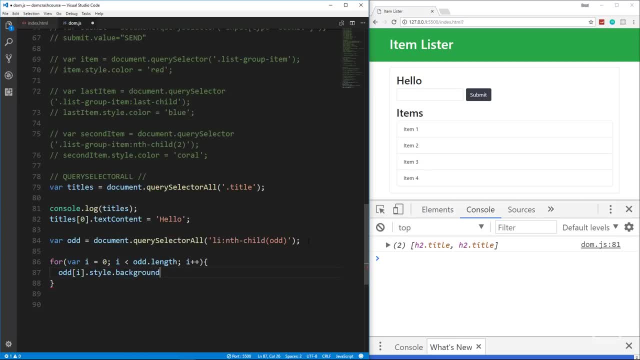 we'll take the current iteration and we'll say dot style dot, say dot style dot, say dot style dot. background color, background color, background color and we'll set that to light gray and we'll set that to light gray, and we'll set that to light gray and save. and now every other one is. 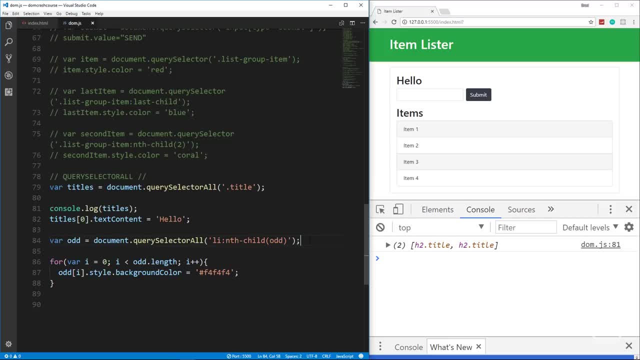 and save, and now every other one is and save, and now every other one is light, gray, light, gray, light, gray. all right, if we wanted to do even. we all right. if we wanted to do even we all right. if we wanted to do even, we could go ahead and 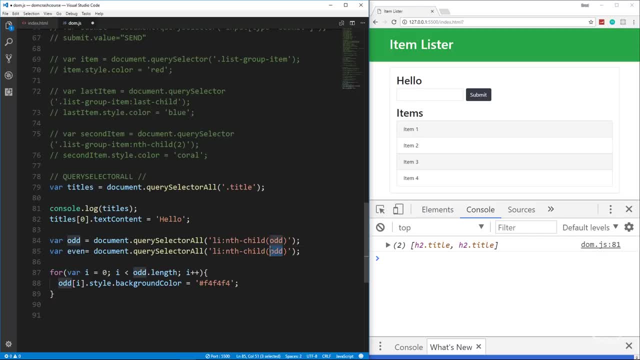 could go ahead and could go ahead and set this to even, and then for the set this to even, and then for the set this to even, and then for the selector we'll just do nth child even and we'll go ahead and copy that let's say even and we'll change the. 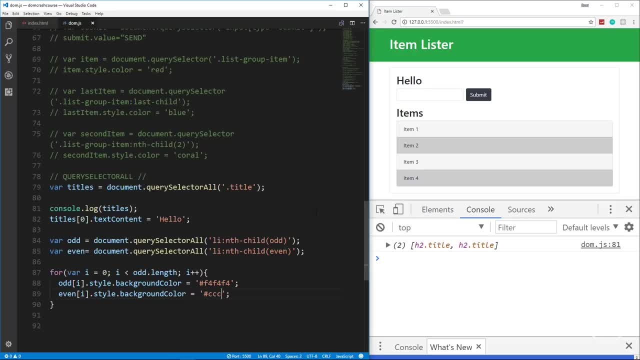 let's say even, and we'll change the. let's say even, and we'll change the color. let's say to a darker gray color. let's say to a darker gray color. let's say to a darker gray. and there we go. all right, so we can do. 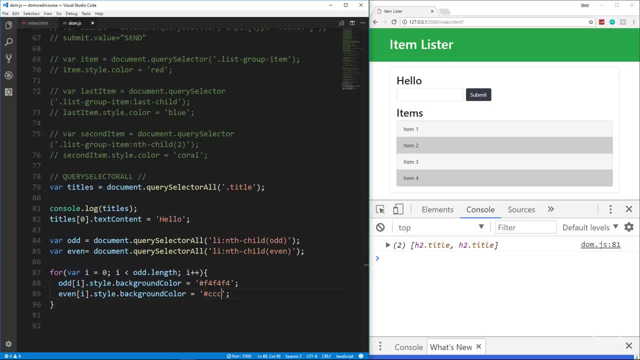 and there we go, all right, so we can do. and there we go, all right, so we can do things like that in vanilla javascript, things like that in vanilla javascript, things like that in vanilla javascript, pretty damn easily, pretty damn easily, pretty damn easily. all right guys. so i'm realizing that i 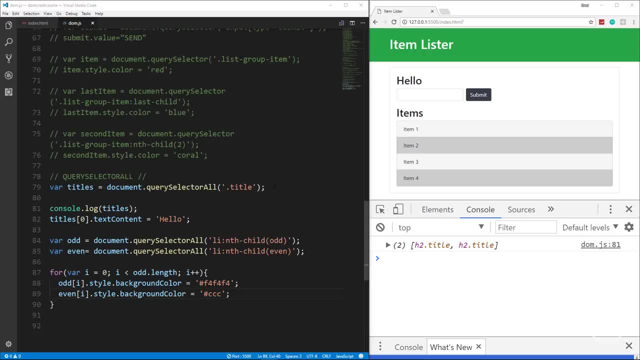 all right guys. so i'm realizing that i all right guys, so i'm realizing that i still have quite a bit that i want to still have quite a bit that i want to still have quite a bit that i want to cover, cover, cover. we went over all the selectors, so i we went over all the selectors, so i we went over all the selectors, so i think that this is going to be a good think, that this is going to be a good think, that this is going to be a good place to stop for this video. place to stop for this video. 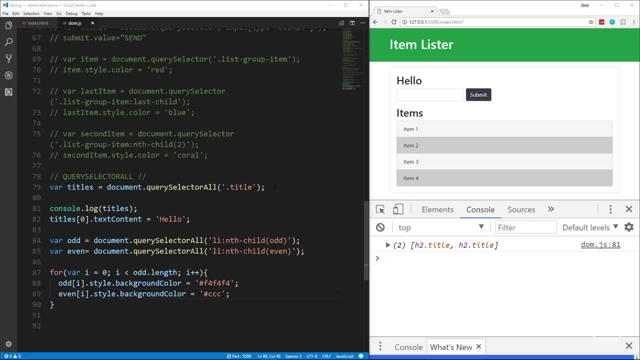 place to stop for this video and we're going to have to turn this, and we're going to have to turn this, and we're going to have to turn this into a little series, into a little series, into a little series. maybe one or two more videos, because i 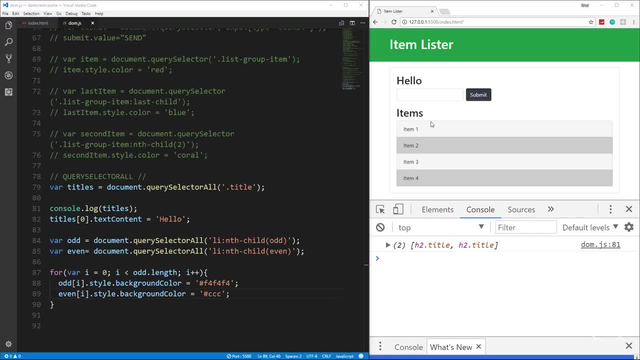 maybe one or two more videos, because i maybe one or two more videos because i want to get into traversing the dom, want to get into traversing the dom, want to get into traversing the dom. i want to show you how we can move like. i want to show you how we can move like.